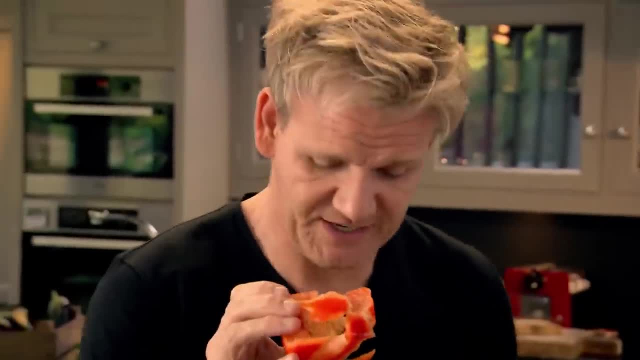 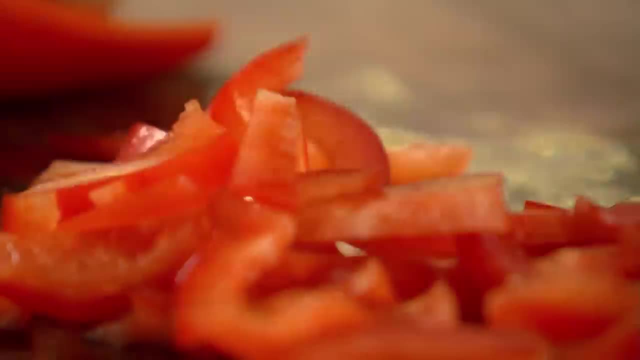 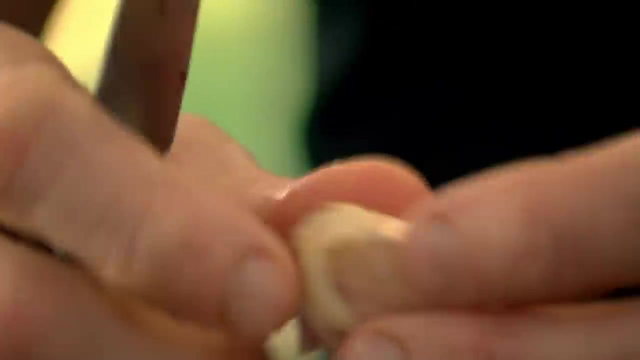 I want to see that sort of little core, Those pips in the centre. No fine diced pepper. The rice is going to be cooking for 20 minutes, so I want the veg to sort of have texture after it's. cooked. Peppers in A bit of garlic, Two nice cloves Just slap down Off with the shell. 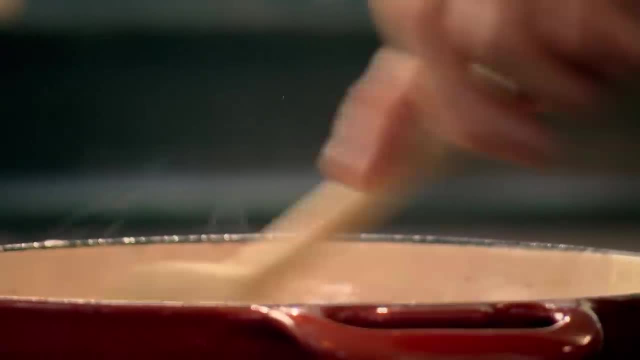 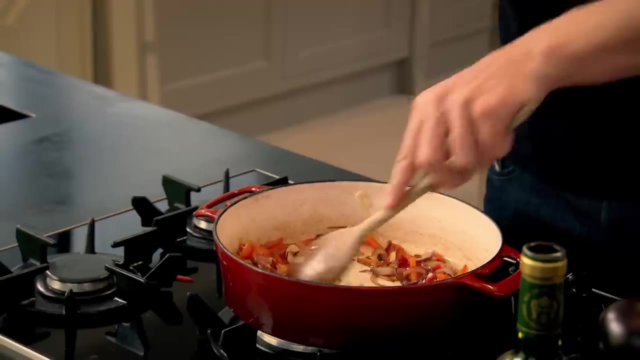 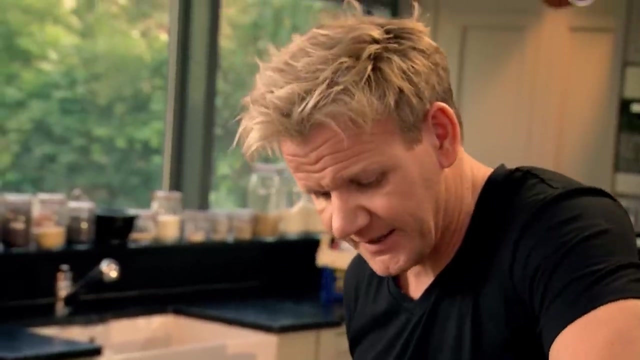 Garlic in. Now I want to turn up the gas, Get the pan nice and hot, because the minute that sausage goes in, everything cools down and you'll end up boiling the peppers and the onions and the garlic. So heat up to maximum and then just make a well in the centre In. 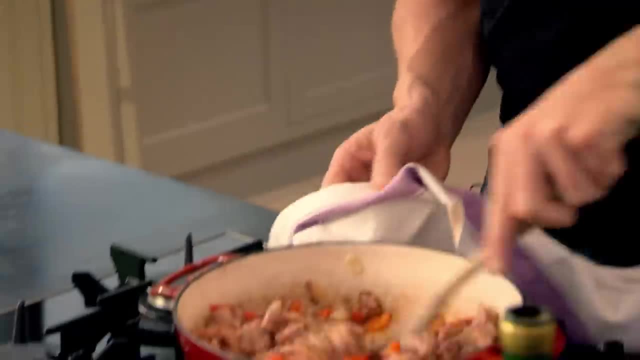 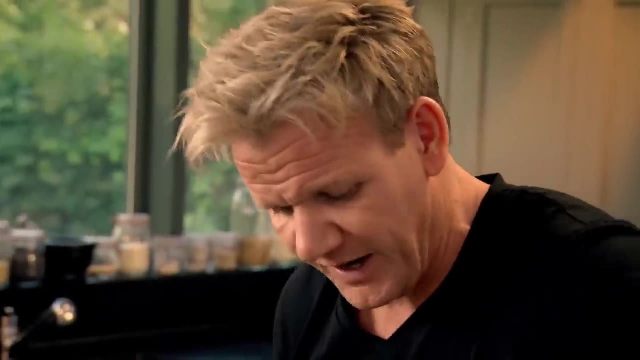 Now start stirring quickly. This is where you get so much more bang for your buck out of sausages, because the skin's off and the real flavour of that- The spicy Italian sausage- is going to come through. What's great about this recipe is: 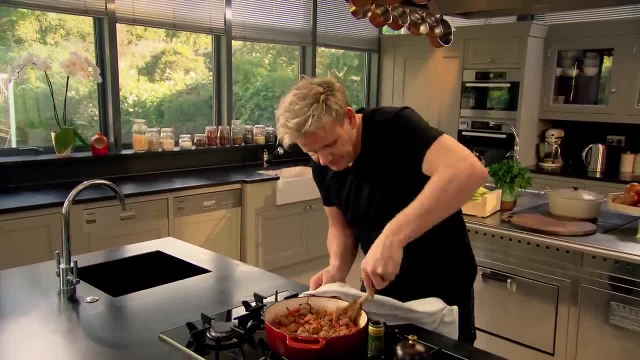 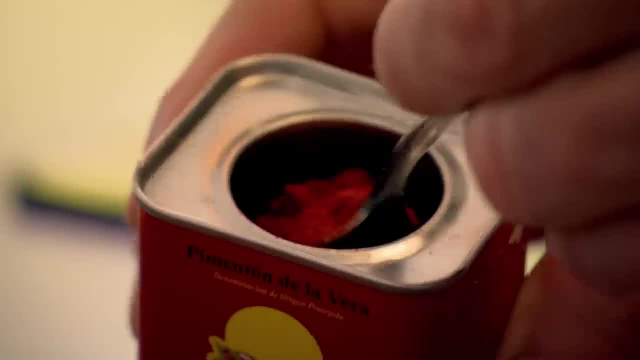 that you can use any type of sausage to get the flavor and the heat you want. I've gone for the spicy Italian, but it's just as good with merguez or chorizo. A teaspoon of paprika in Give it that really nice smoky flavor. 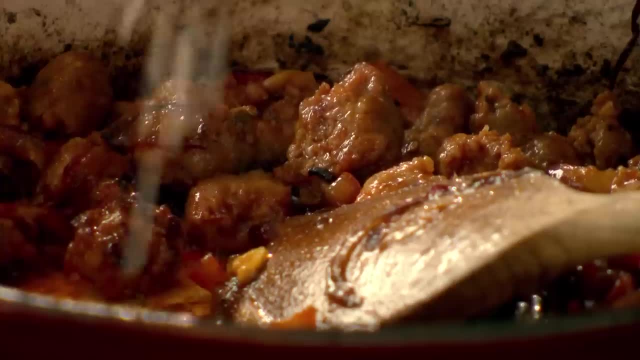 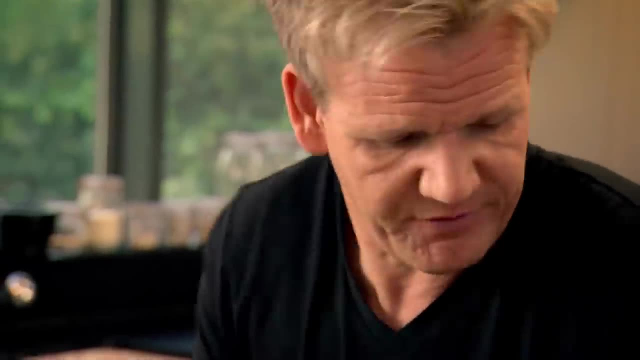 Rice in And we're going to sort of basically sear the rice- We call it in the kitchen blasting the rice- where we sort of sauté the rice for 30 seconds And it takes on all that flavor. Next, white wine. 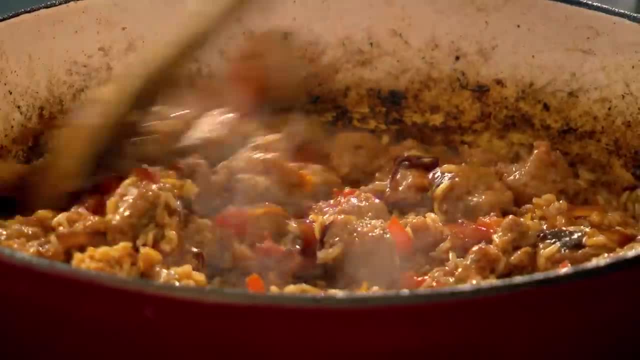 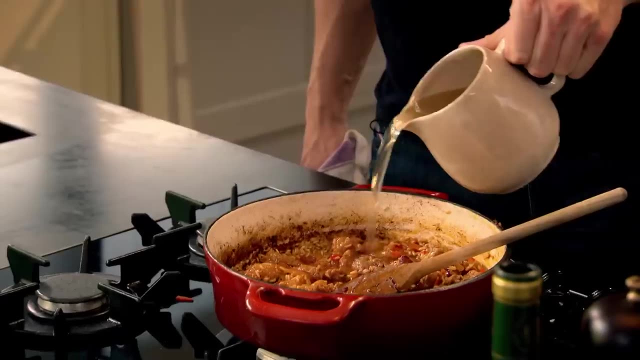 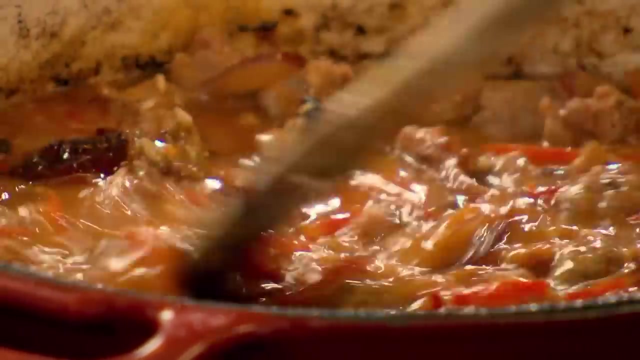 So the wine sort of deglazes the pan and washes all that flavor from the bottom of the pan into the rice Stock in. Bring it up to the boil, Turn it down and let it simmer. Double stock to rice, Turn that gas down and let it simmer for 12 to 15 minutes. 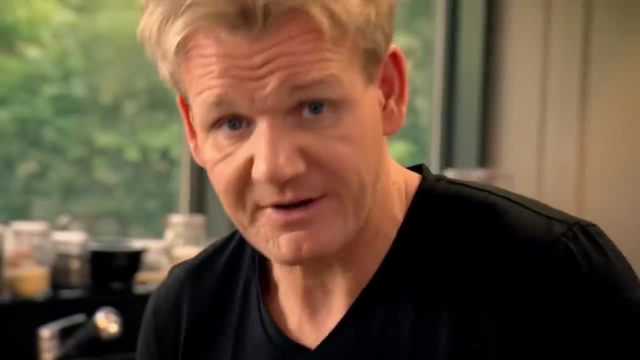 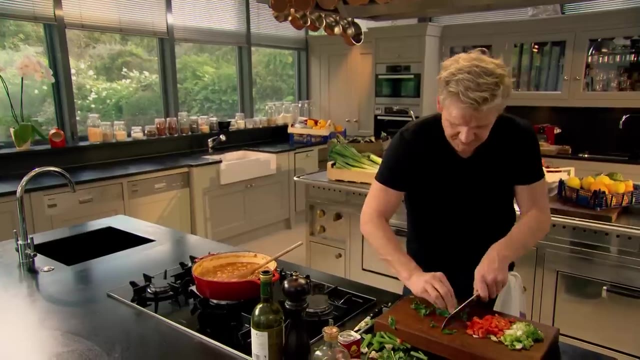 And done. Just give it the occasional stir. Keep an eye on it. Now get ready to finish it. Sliced spring onions, diced sweet juicy tomatoes and roughly chopped earthy flat leaf parsley. Spring onions in Tomatoes in. 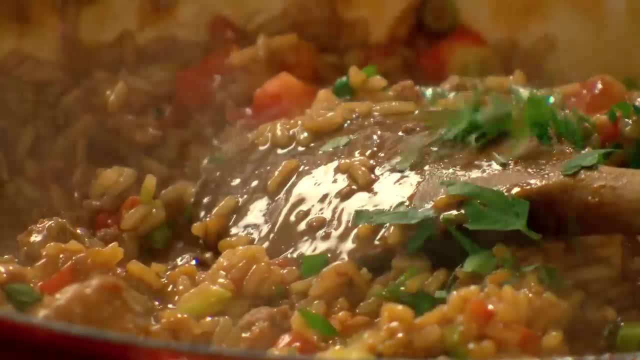 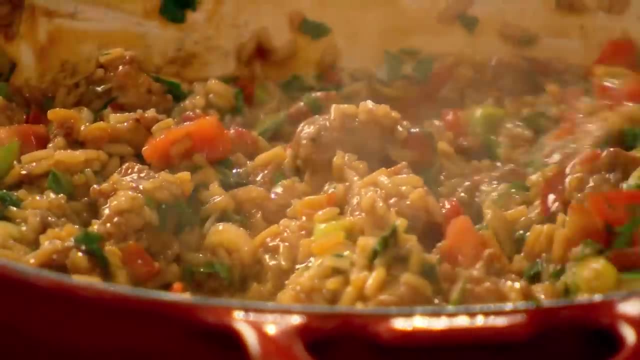 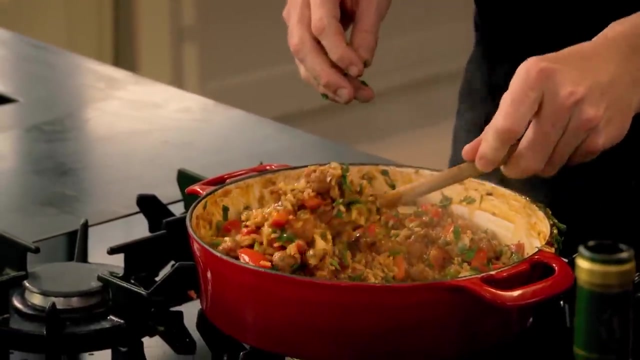 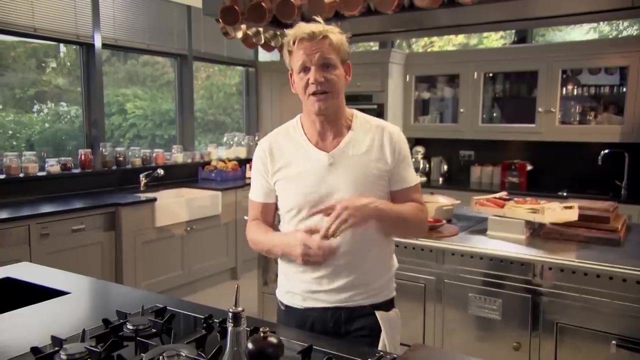 Off with the gas, Really important. Otherwise everything becomes overcooked. Flat leaf parsley in. But look at the volume in that pan. now That is an amazing way to take spicy Italian sausages to a completely different level. Beautiful. First off, get your pan on and start sweating off. 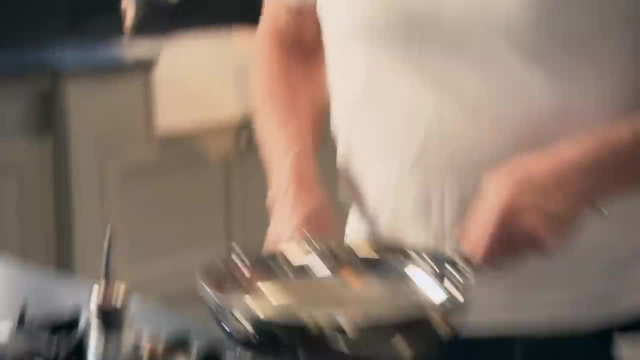 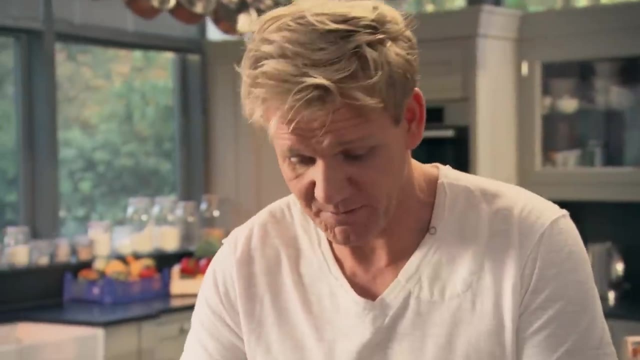 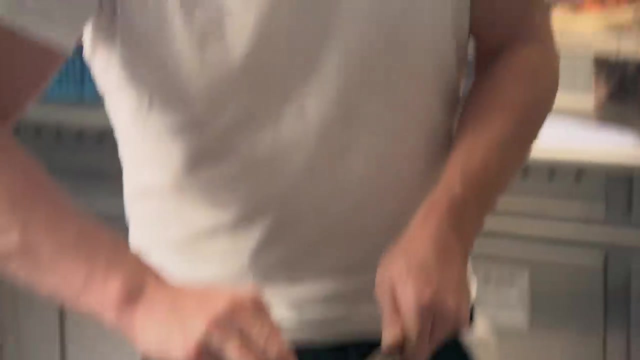 your onions and your garlic. This recipe involves making the meatballs in a classic way, But the exciting part is actually cook them in coconut milk And it gives a really nice new dimension to a sort of soft, rich, sumptuous meatball. 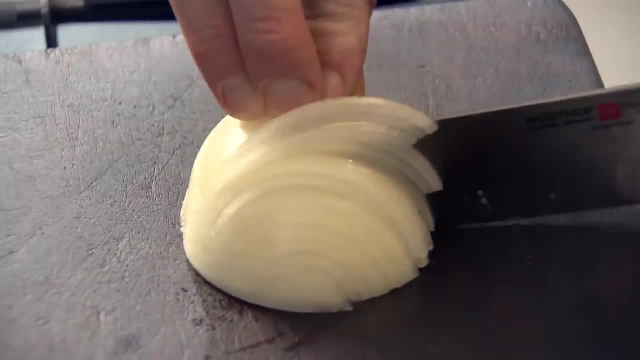 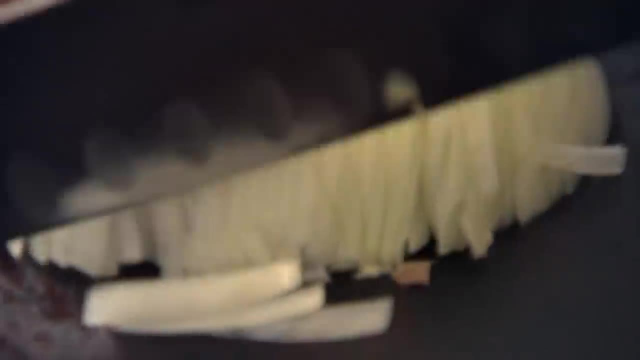 Chop the onion nice and finely, keeping those slices very close together. The closer the slices, the finer the onion. Pat it back down at an angle, Slice down and just chop. I want the onions nice and fine because I want some finesse. 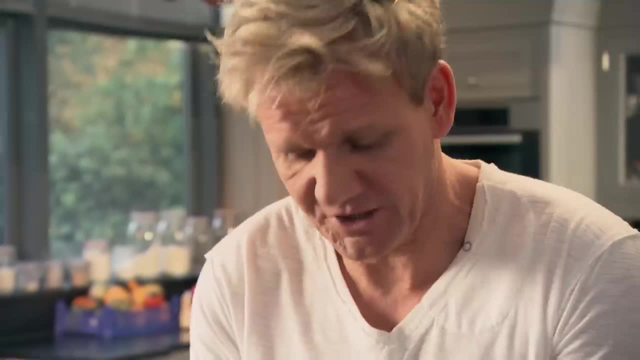 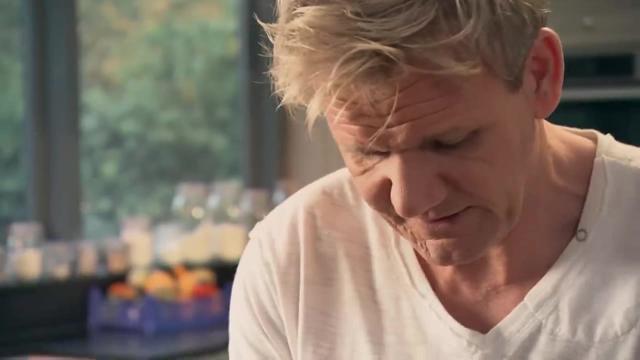 to these meatballs. And the secret of a really good meatball is the texture, getting that balance right between the minced beef, the breadcrumbs, the milk and the seasoning. A couple cloves of garlic: Slice the garlic really nice and thinly. 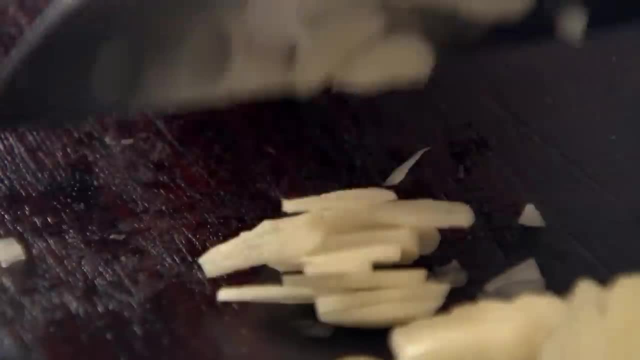 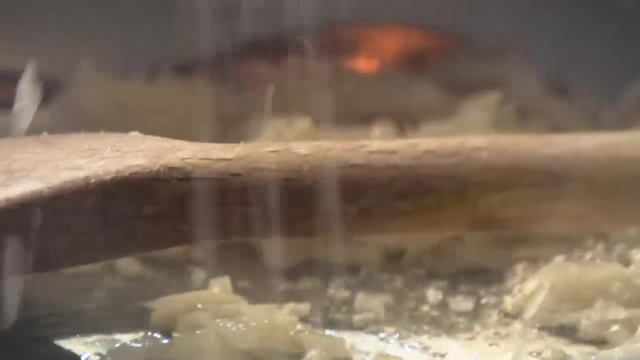 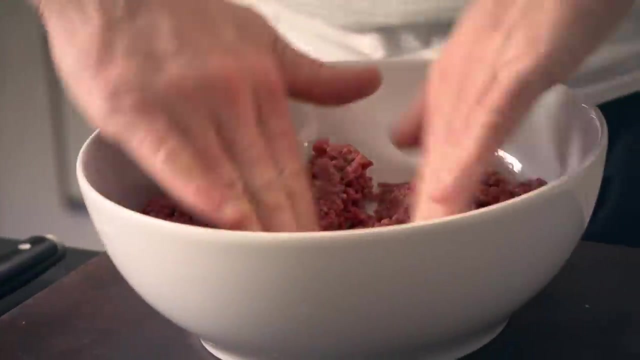 Nice Pan, nice and hot, And a tablespoon of olive oil. Quite generous with the olive oil, Onions and garlic in Little touch of salt and pepper. With your mince, open it up a little bit and sort of pat it out. 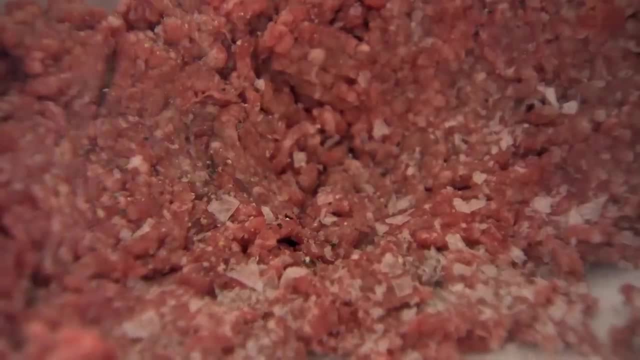 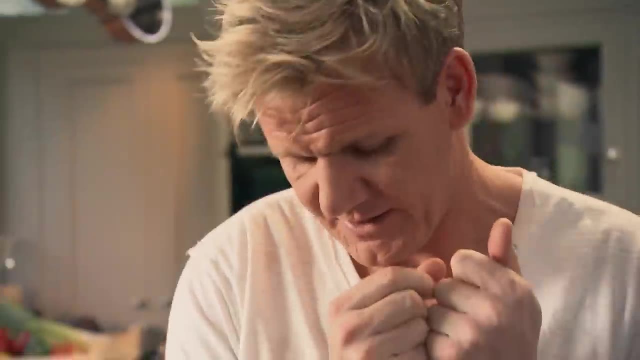 Salt and pepper. For me, a good meatball is all about the softness, the texture of that rich beef And the way it sort of melts in your mouth. You can color it on the outside, but you want it nice and soft. 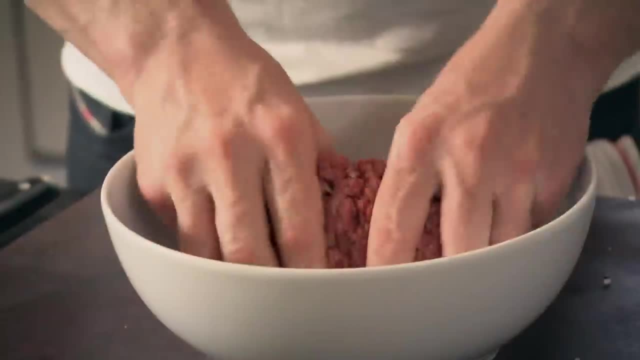 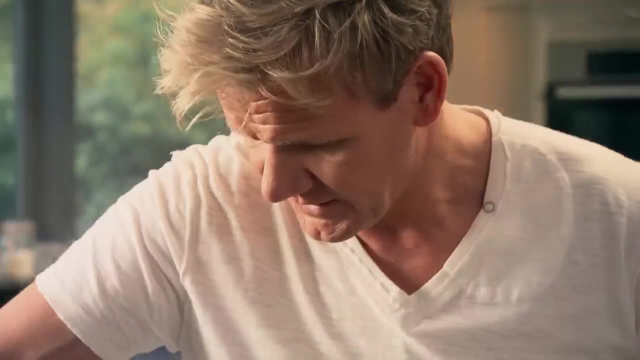 and sort of rich in the center. Mix that in beautifully And then paste it back out again. I've got some really nice dried chili flakes. I'm going to season the onions with the chili flakes, Chili flakes in. Cook that out for two minutes. 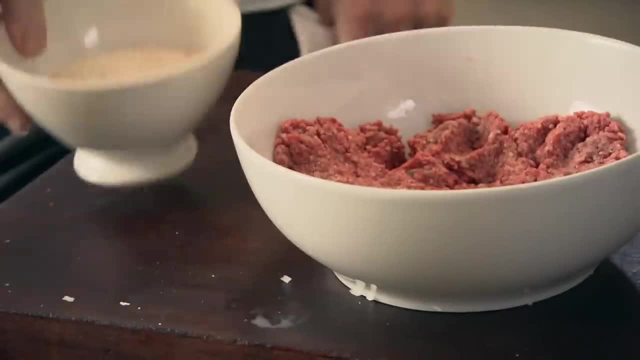 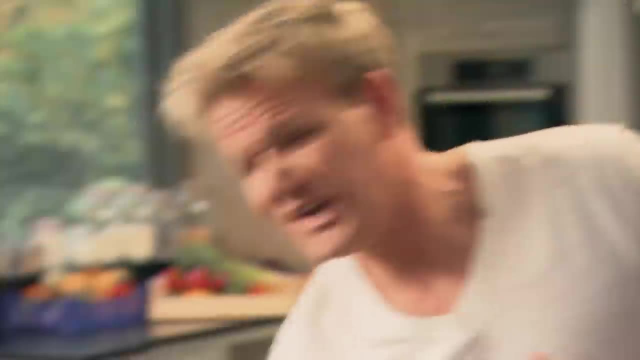 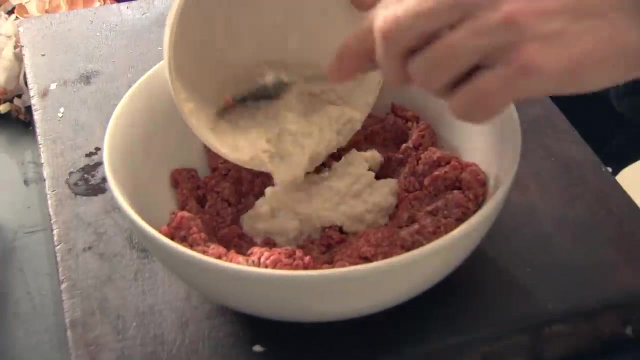 I'm going to add some milk. Take your breadcrumbs, Make a little well, Three or four tablespoons of milk. That makes a sort of nice, slightly doughy texture, But it lightens the texture of the meatball. Place that in. 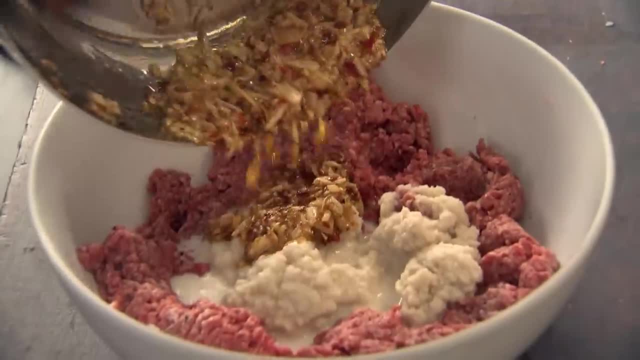 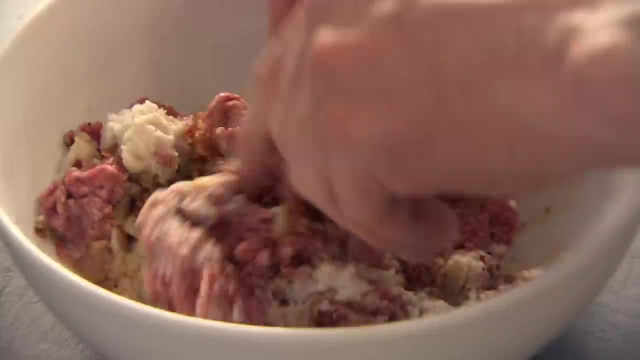 Add your onions, your garlic and your chili in there as well. Nice, Get your hands in there and start mixing them If you've got the right amount of milk and breadcrumbs. it doesn't mean binding with an egg. Don't make them too small. 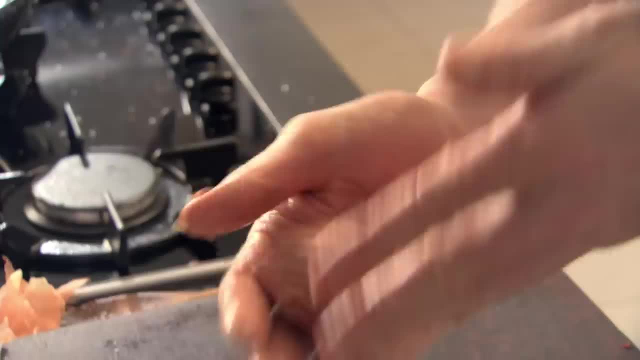 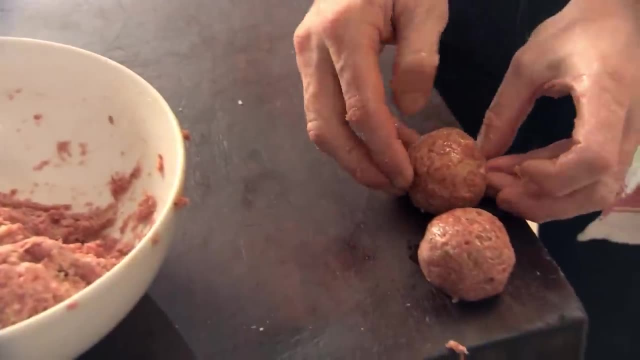 The problem with making them too small is the fact that they dry out quickly. Just the size of a golf ball, A little bit bigger, Nice. Give them a really nice tight squeeze That stops it from breaking up. It always pays to double the recipe. 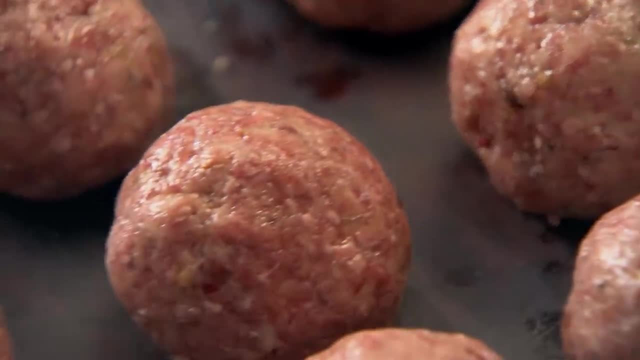 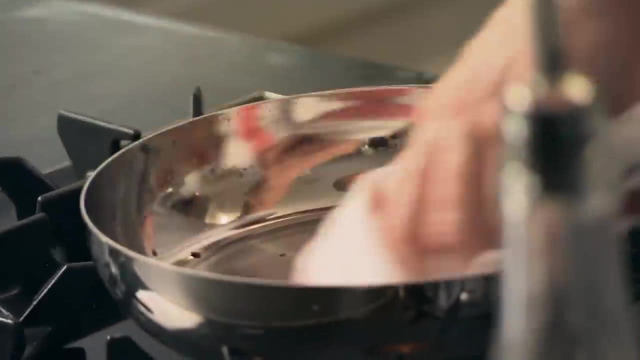 and spend a bit more time making extra meatballs so you can freeze a batch ready for another time. Give the pan a little wipe out, Don't wash out that pan. We've got that flavor from the onions and the garlic at the bottom. 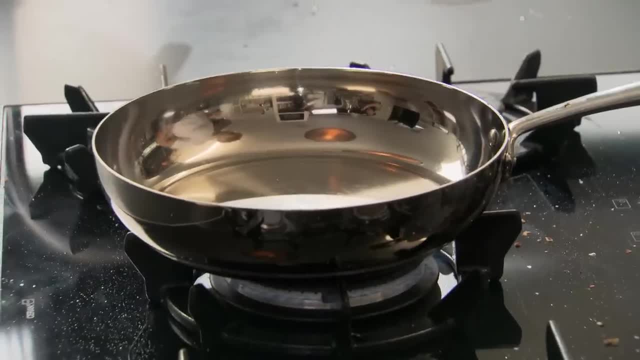 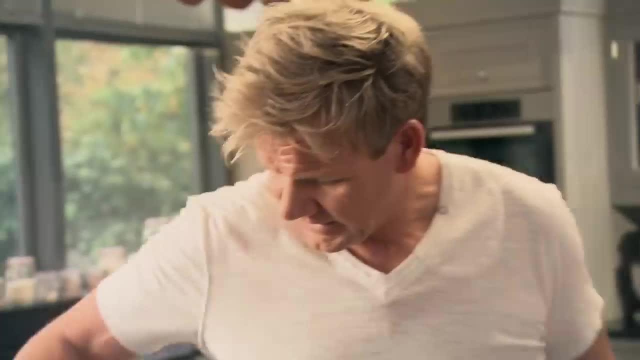 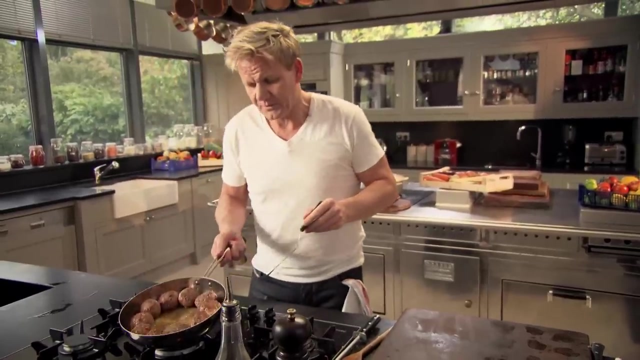 Get that pan nice and hot A touch of olive oil in there, Just like that. Place them on the top of your pan, Nice, and gently sit them in the oil. Get a palette knife and go underneath them and just sort of tilt the pan and let the pan 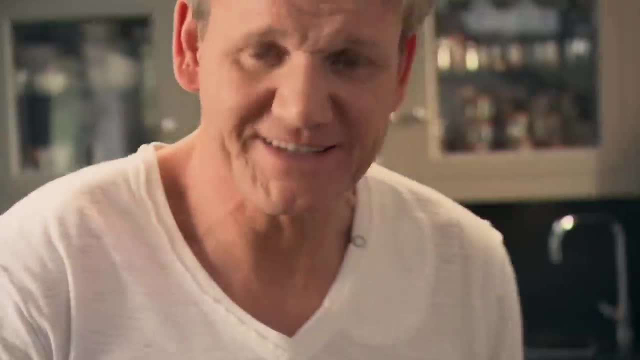 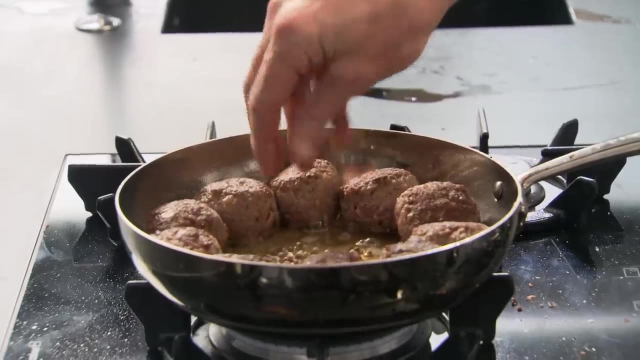 cook the back of the meatball. We're going to add some heat. Coriander seeds, Slightly spicy and peppery. This will give a really nice flavor to the coconut milk. In Next, some cardamom seeds, Three or four onto the board. 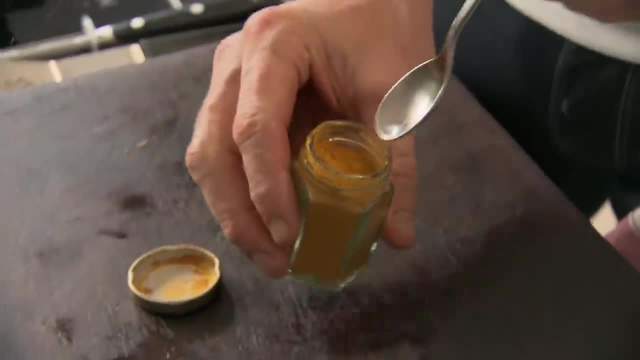 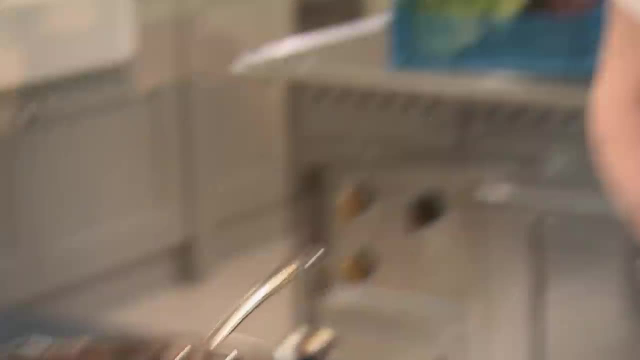 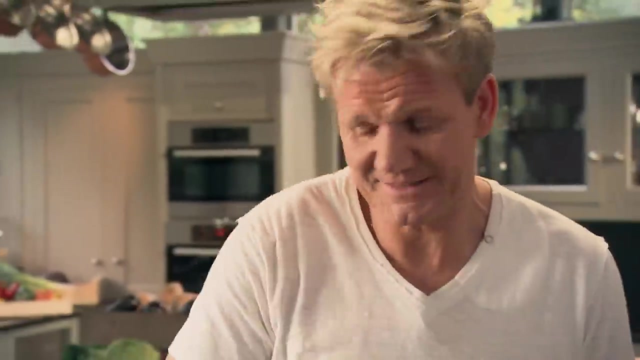 Knife on In A little touch of turmeric into the center of the pan. That's going to give it a really nice spicy flavor. A little pinch of cinnamon. All the time you're doing this, those meatballs are just getting tastier and tastier. 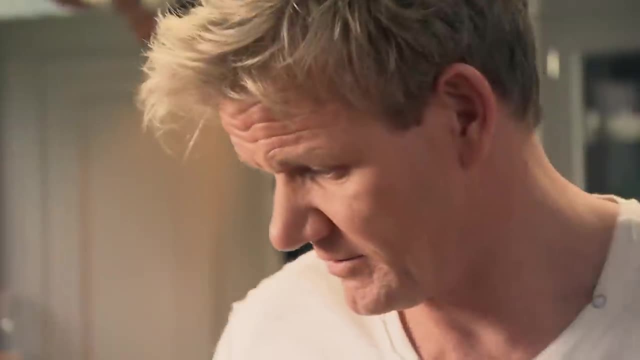 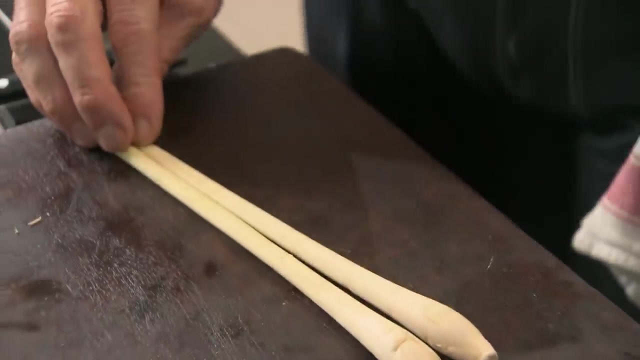 A couple of dried chilies, Let them infuse in that oil, And then some lemongrass. Just take the back of your knife and sort of beat it down. That starts to release all that. you know that flavor, All that lovely sort of fragrance. 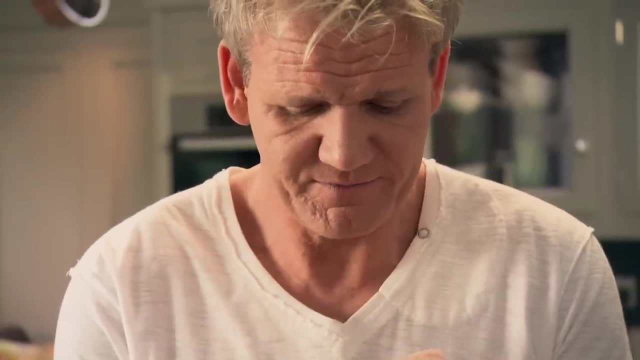 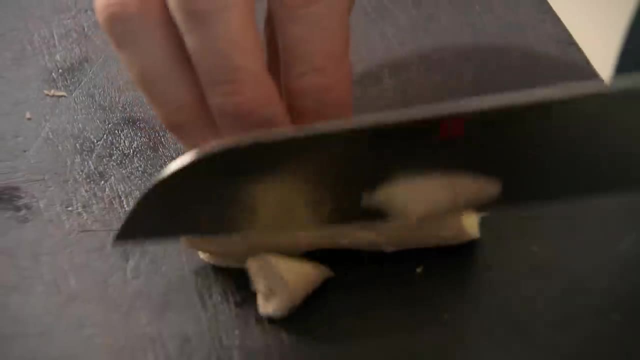 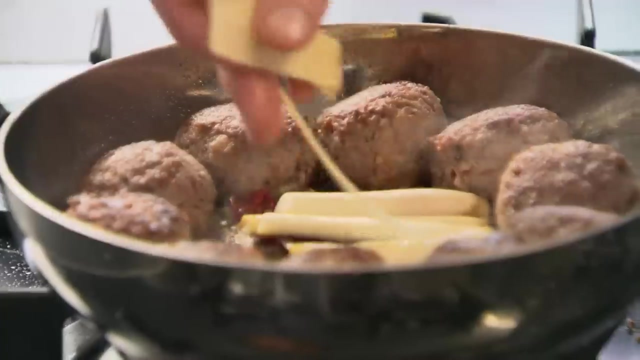 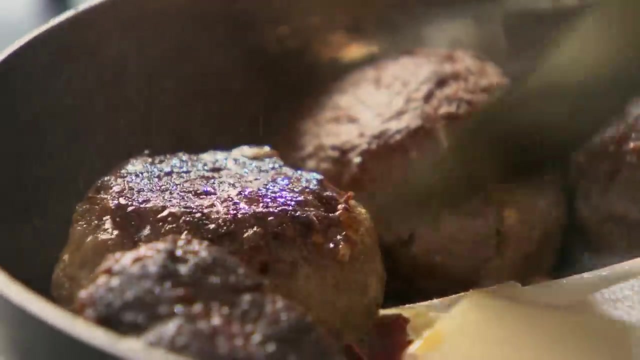 Like someone's just let off the most amazing fragrant air freshener. In with the lemongrass And finally some fresh ginger. Just peel and slice nice and thinly. Time now to turn them over And let the other half have that wonderful flavor. 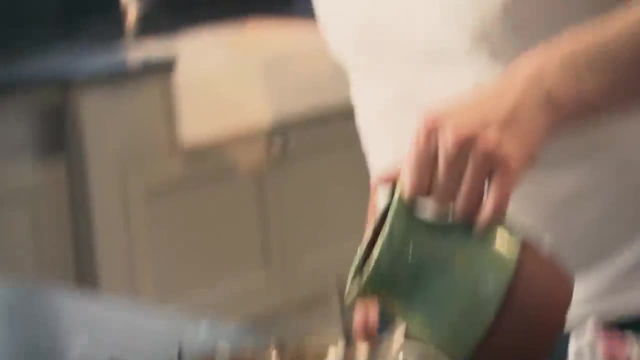 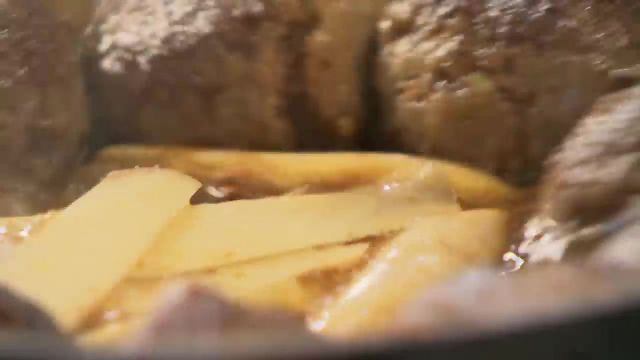 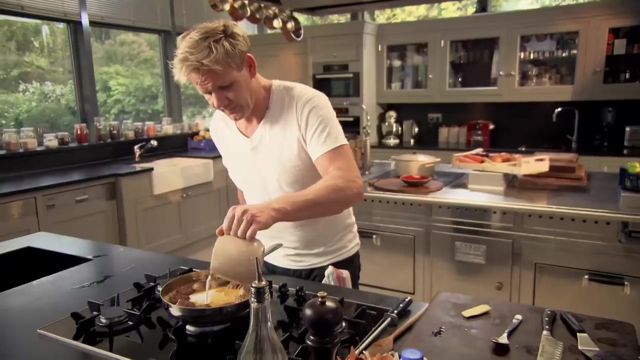 Chicken stock In. Bring the stock up to the boil, Turn the gas up And then add the coconut milk And I want the coconut milk just sitting underneath the top of the meatball- Coconut milk in And that sort of gives it that creamy richness, but it's not heavy. 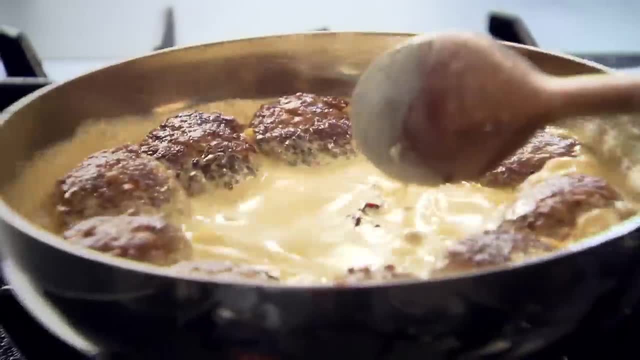 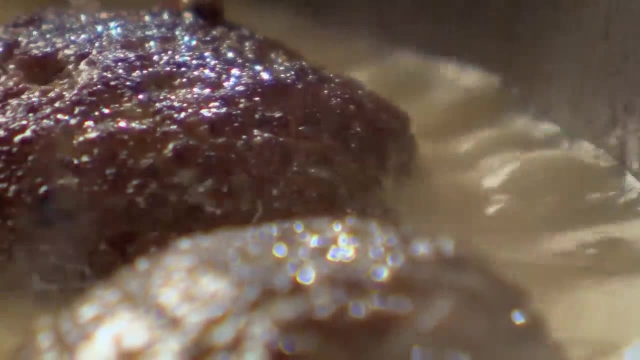 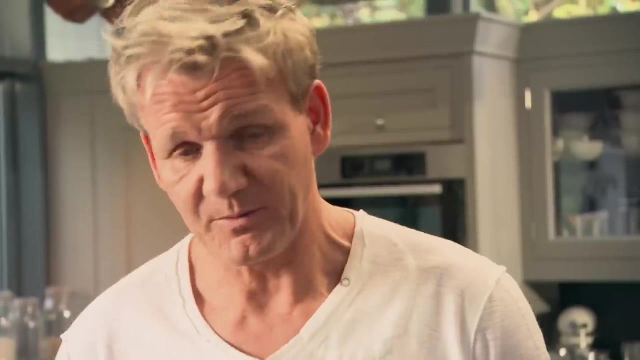 It's a fragrant, light richness. Before we start simmering, Check the seasoning. Mmm, That nice soft texture of the meatball, But that fragrance, light richness of the coconut broth is going to cook those meatballs perfectly. 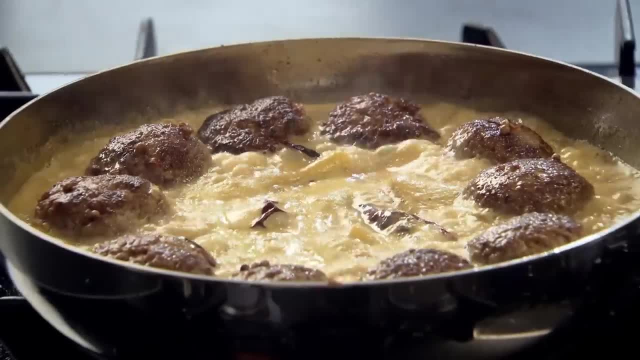 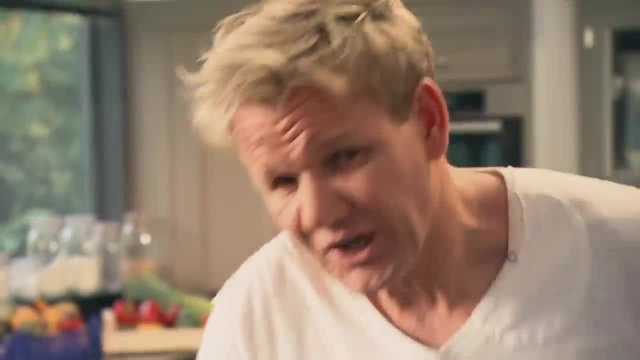 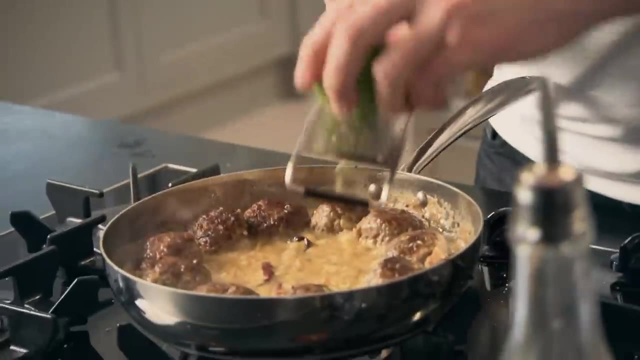 Bring the broth up to the boil, Then simmer gently for eight to ten minutes. Touch them with your finger. This should be slightly pliable, but slightly springy. Gas off. I'm going to finish it off with something light and fresh. 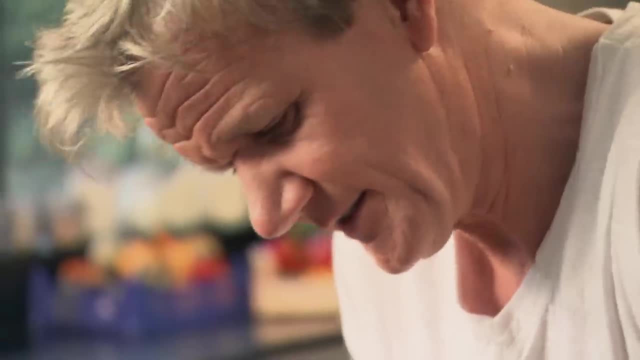 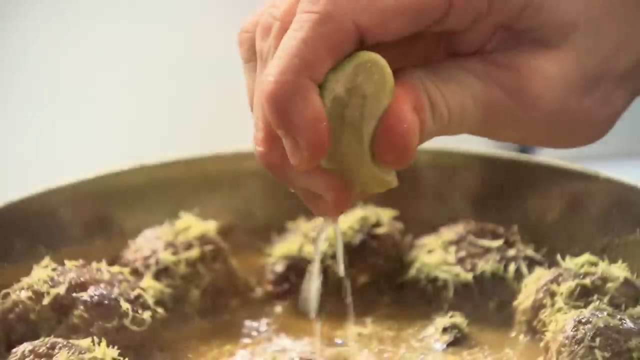 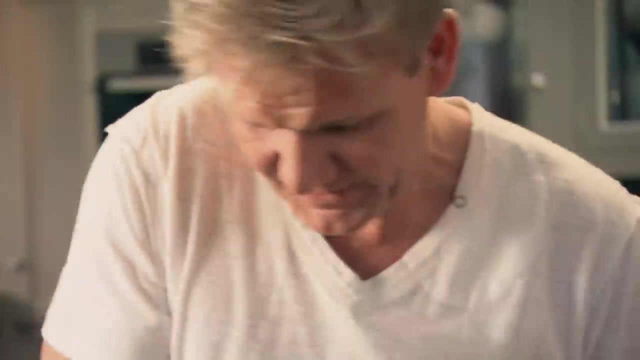 Zest of lime, But I want the zest on top of the meatball, Sort of cut through that richness, And then finally squeeze the fresh lime And that just gives it that nice, zesty, amazing taste. Stir in the juice. 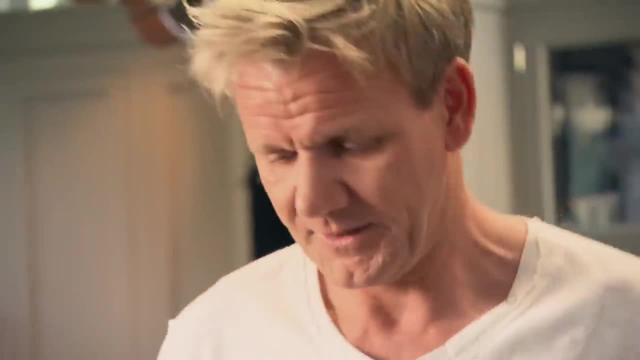 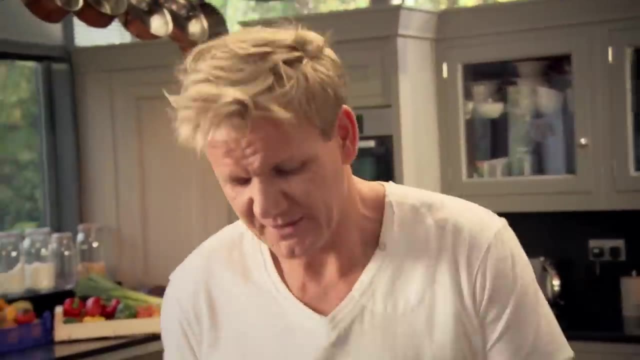 Mmm. It's got that kick and that vibrant taste. Now the exciting part: When you come to serve it, be generous with that coconut broth. Tilt the pan, Get a good couple of ladles of the broth in Mmm. 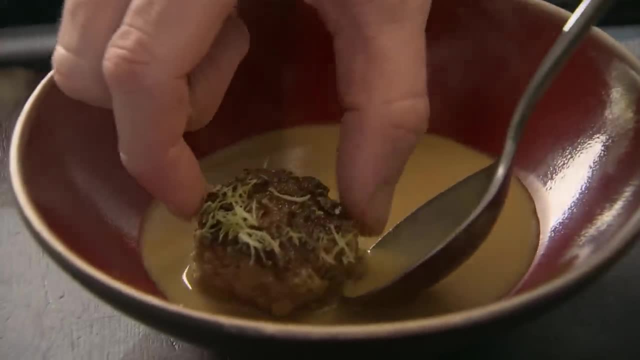 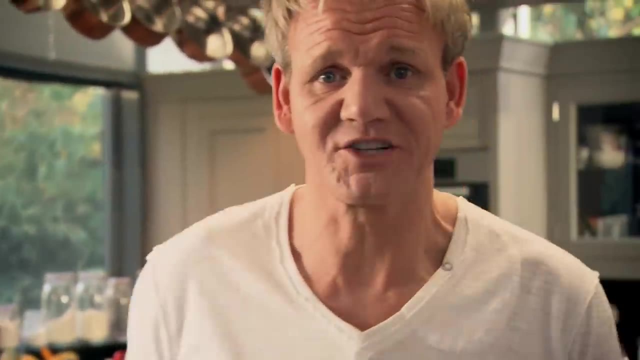 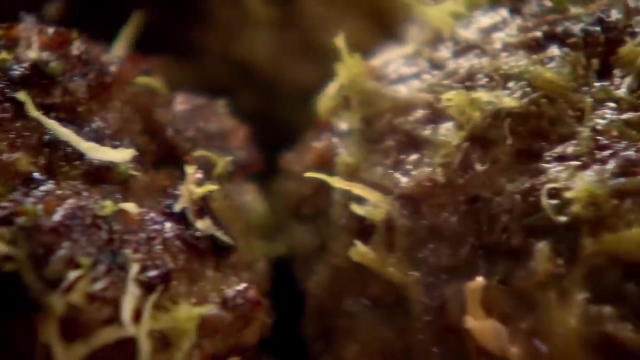 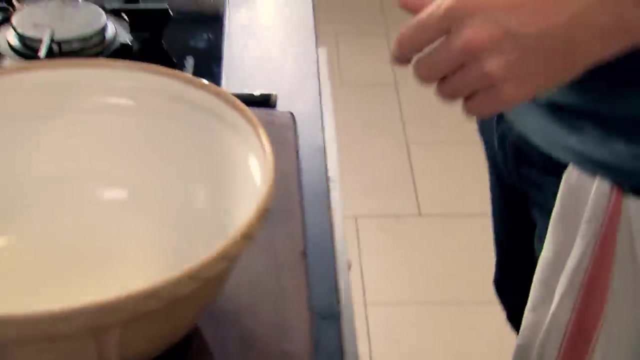 Meatballs, And that is a very delicious way of eating an old-fashioned meatball and bringing it into the 21st century. And they're just as good cooked from frozen as well. Take a sieve. When you think of shortcrust pastry, it's sort of semi-flaky, but it's rich, buttery. 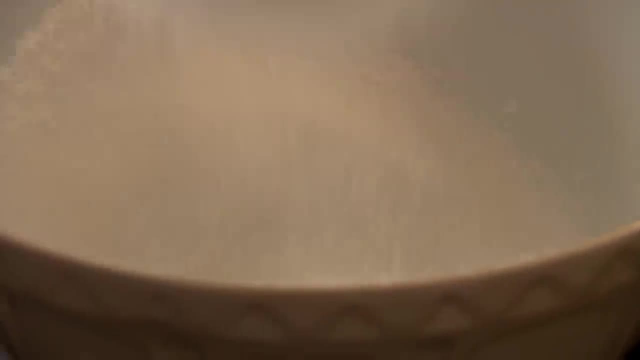 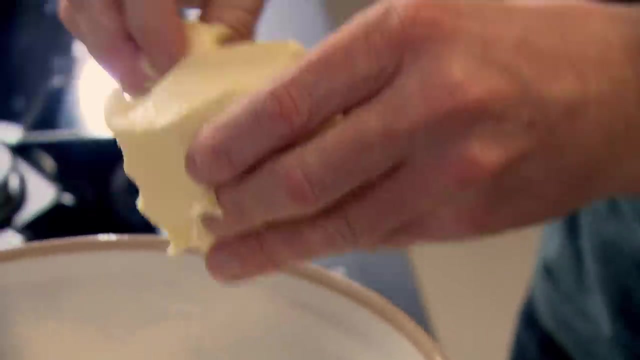 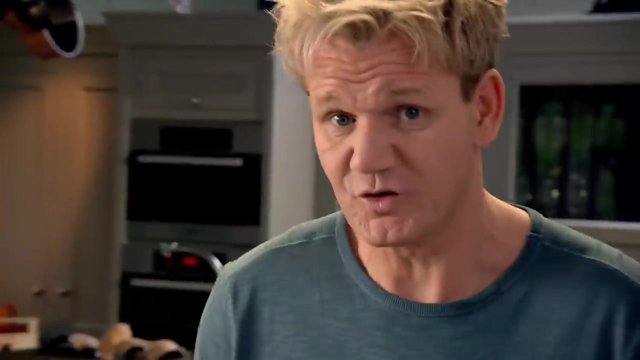 Start by sifting 200 grams of plain flour into a mixing bowl. Large pinch of salt, 200 grams of unsalted butter. Bring the butter up to room temperature. If you let the butter become too soft, then the flour sort of doesn't absorb it. 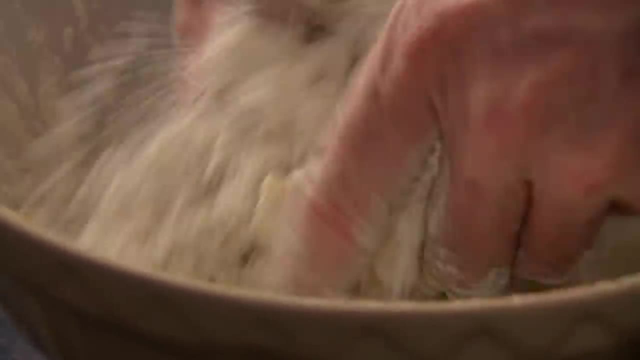 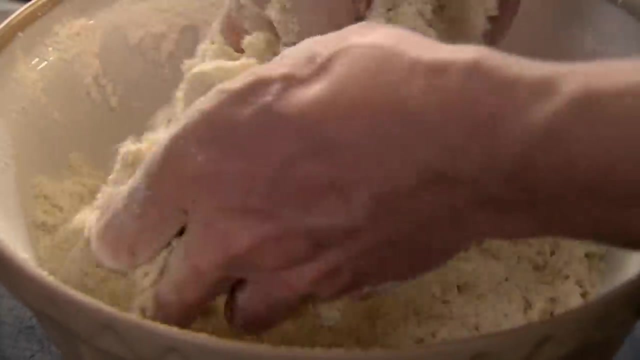 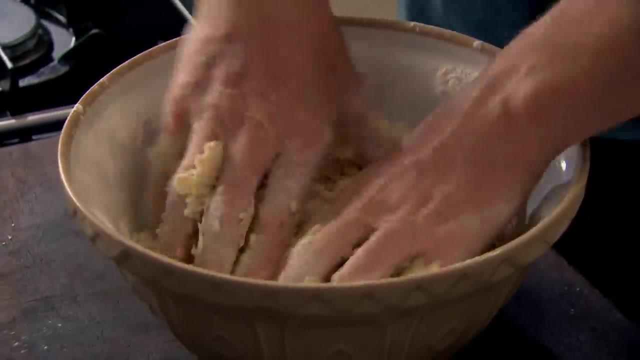 In with your fingers, Rub together first. Now the secret is: grab big handfuls and squeeze the butter into the flour. So look what's happened. Literally in 30 seconds I've got that nice crumbly texture. Now a couple of tablespoons of water. 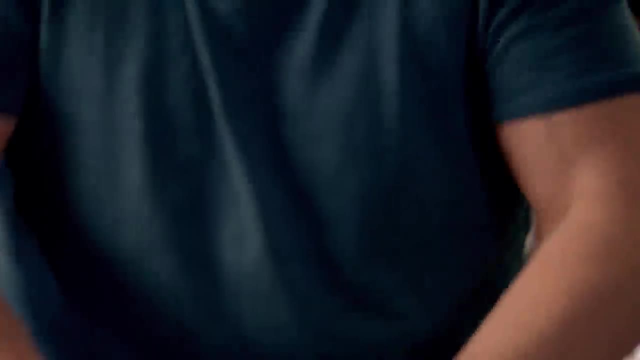 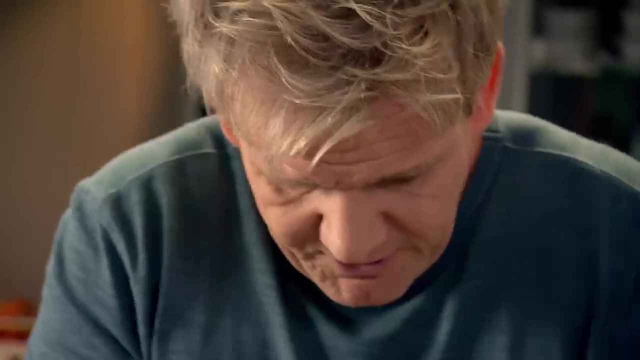 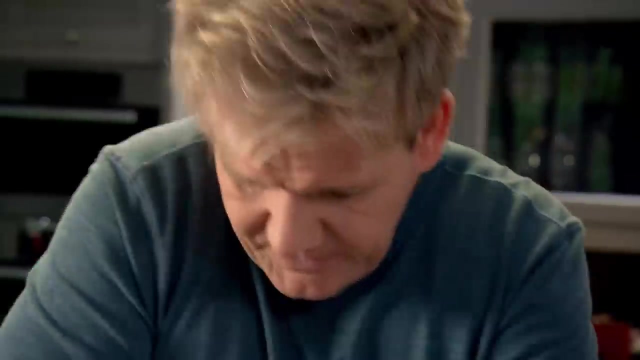 Nothing worse. when the pastry's so wet you can't bring it together. It needs to shape like a nice rich cookie dough And it's just a touch too dry. So one more tablespoon of water And there you go. It's coming nicely. 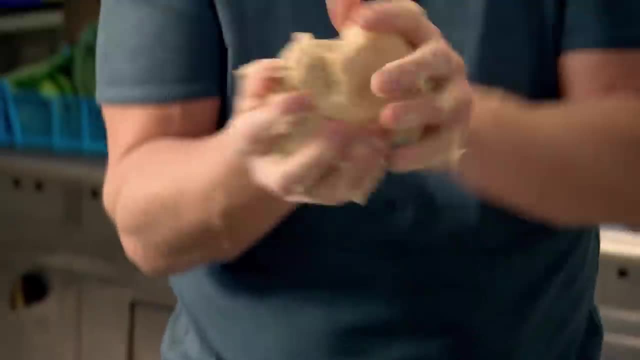 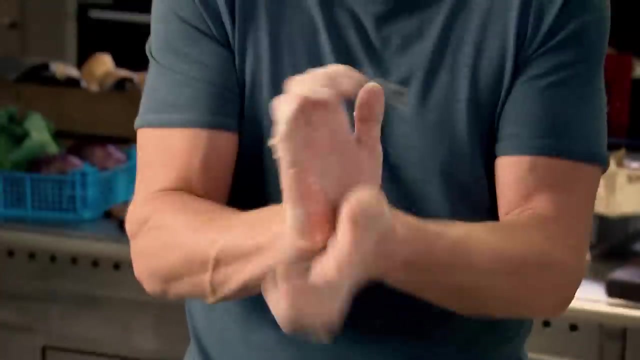 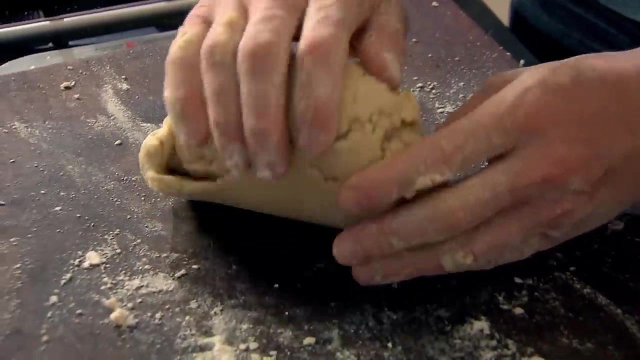 Now, that's what I want: A nice sort of firm ball of pastry Onto the board. We're going to use these, One of the strongest parts of the body, Pull towards you and push back down, Use those hands, Use those wrists. 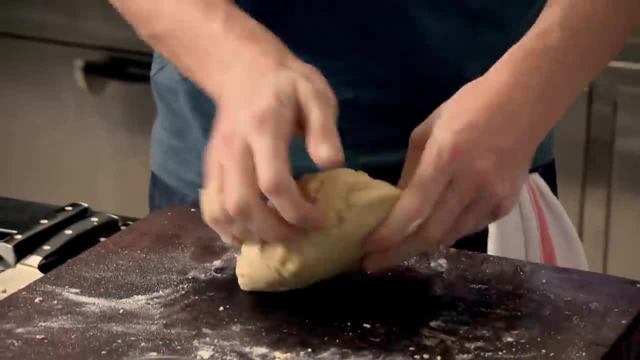 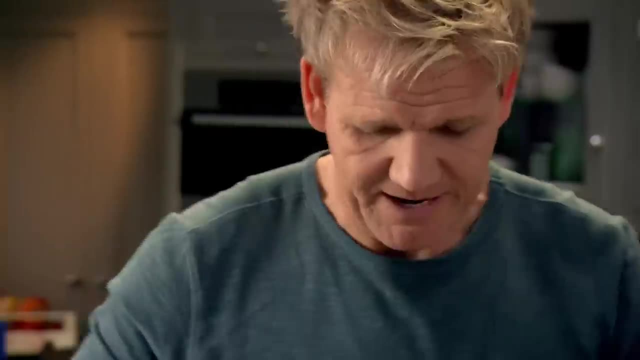 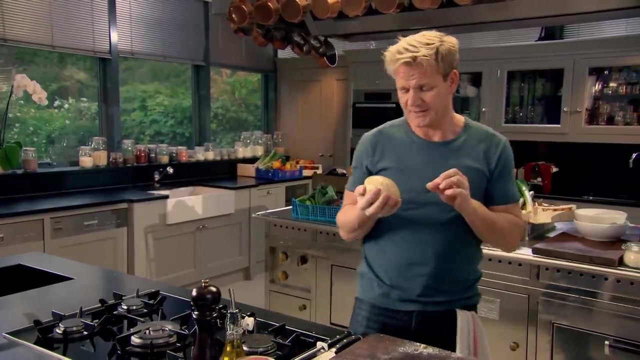 It's really needed Together. So just that nice sort of smooth texture. Now wrap it in cling film. Set that in the fridge for 20 minutes. Really important that you let the shortcrust pastry relax Now to make the quiche. 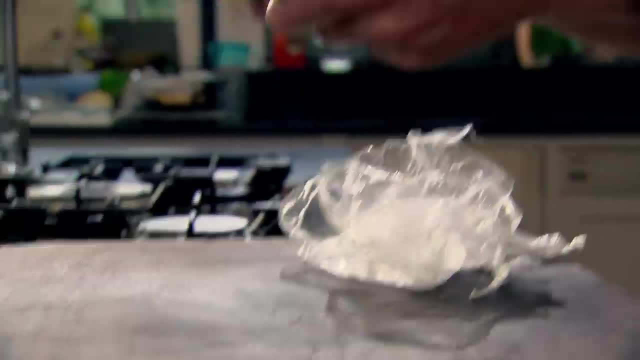 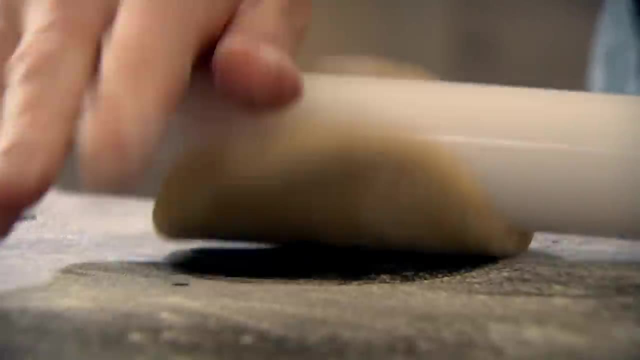 You can use just an ordinary flan dish, but I love making them in mini frying pans, which gives them an extra rustic charm. Brush with oil to stop the pastry from sticking. Once the pastry is at room temperature, roll it out to a nice, even thickness. 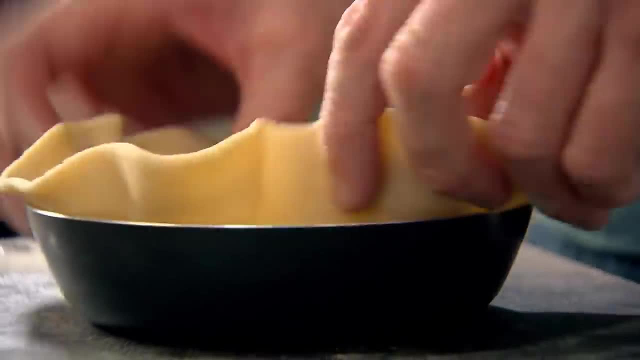 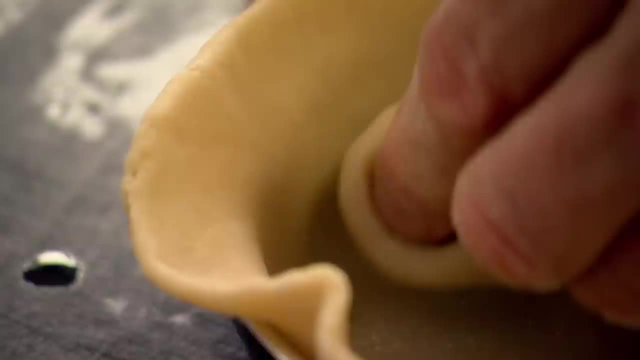 Place it in the center of your little pan, Turn it in. Don't use your fingers, because what we don't want is any holes in this. Just get a little bit of dough, because that sort of acts like a little sort of mallet. 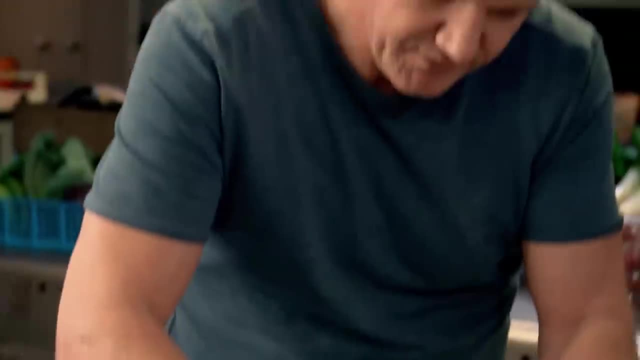 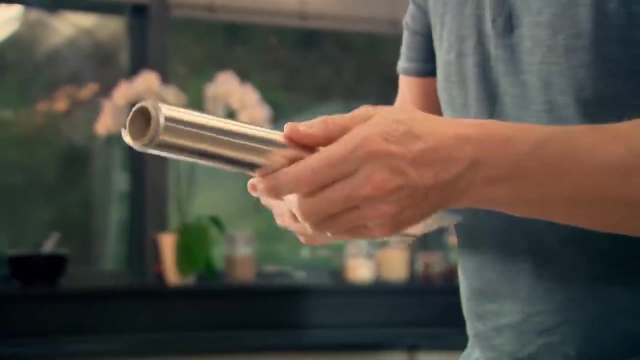 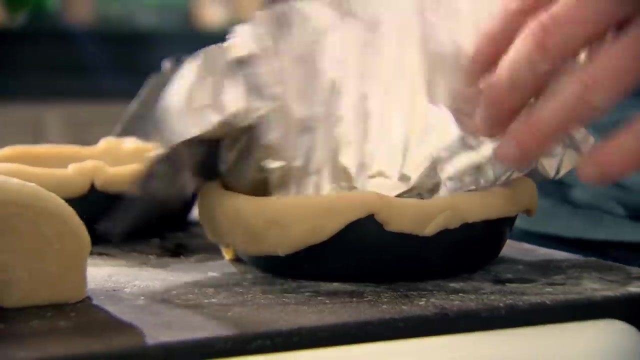 Flattens it out nicely. I'm building a sort of extra lip because that way I can get the filling at its absolute maximum levels. We're going to cook them blind first. To blind bake simply means to precook your pastry before adding the filling. 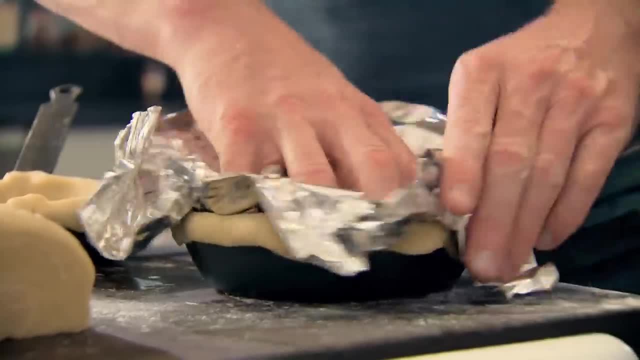 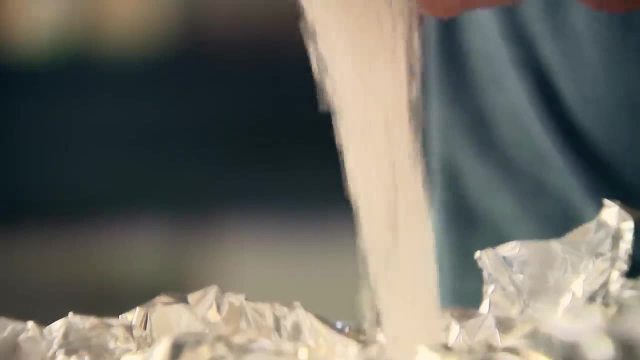 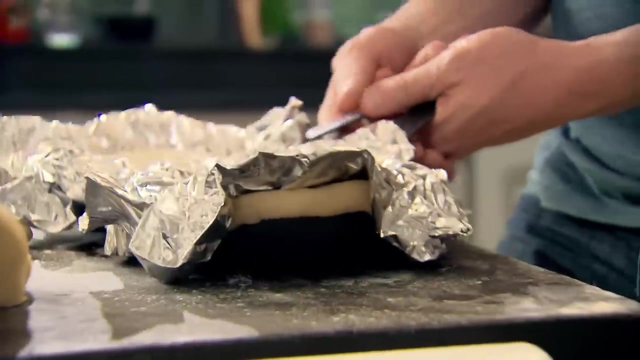 This ensures you'll have a fantastic crisp pastry. Add a sheet of foil or baking paper and weigh it down. You can use rice pulses or ceramic baking stones, Just make sure you keep them for the next time Into the oven, 200 degrees, for 10 minutes. 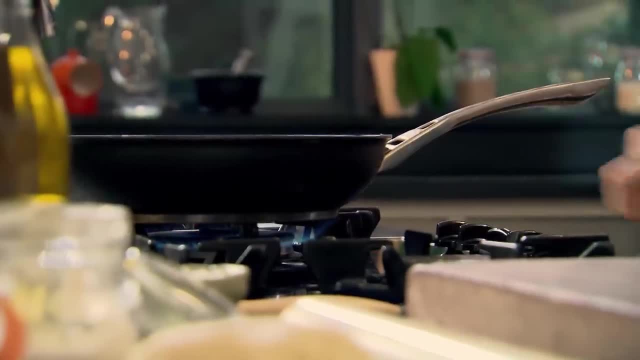 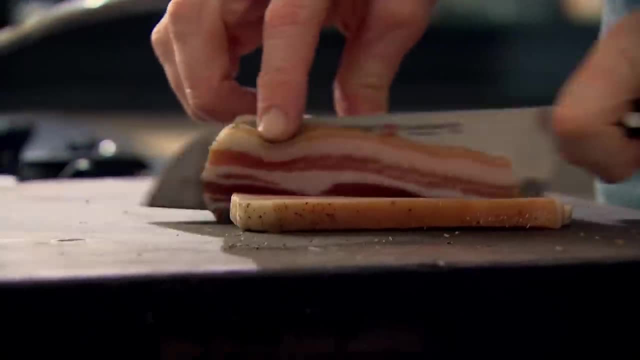 Now for the filling. I'm going to do a classic quiche, Bacon and leeks. This is an amazing cured pancetta. Pancetta is an Italian cured meat made from belly pork seasoned with things like juniper, nutmeg, fennel. 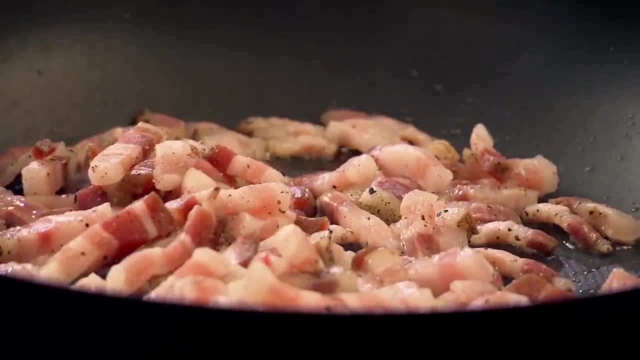 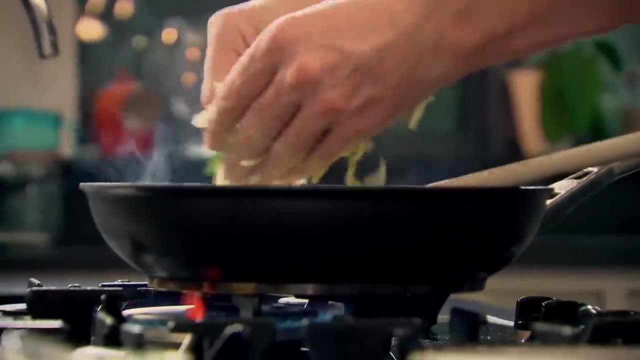 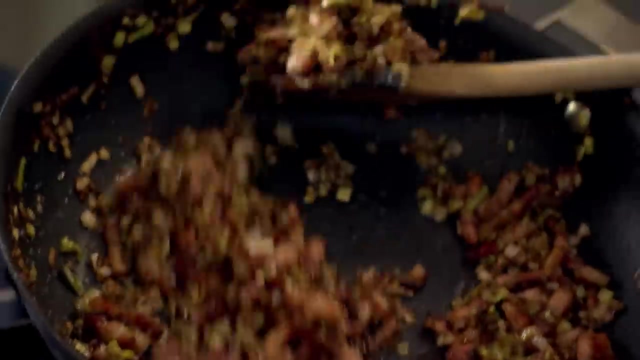 A great substitute is unsmoked bacon. As the pancetta gets lovely and crispy, finely slice leeks and add Whoa Leeks and bacon. Nice, Really important, to cook those leeks down. That's exactly what I want. 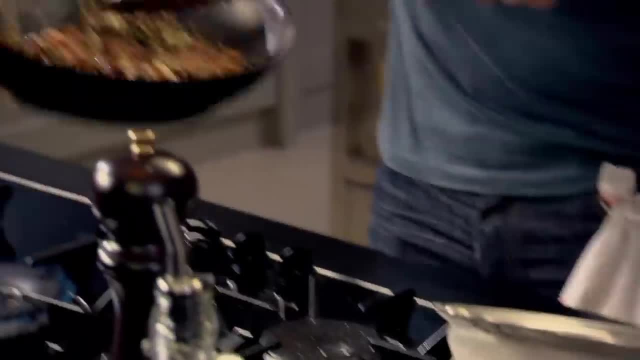 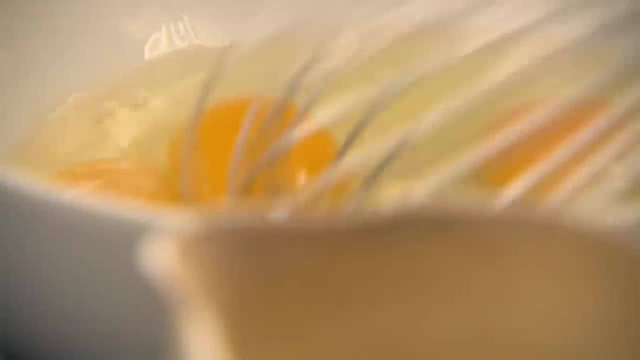 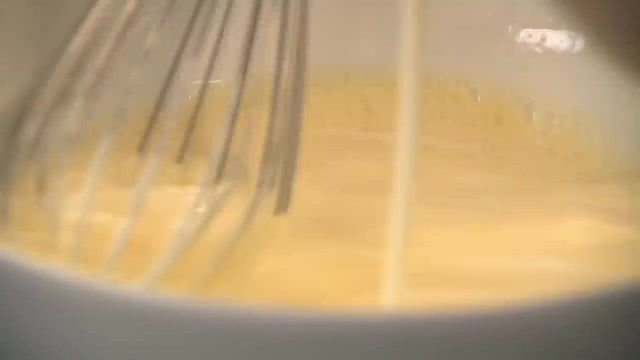 Those leeks are almost sort of caramelised, slightly crispy. The flavour's amazing. I just drain them off so any excess fat gets drained. Couple of tablespoons of cream, It gives it a really nice richness. I want two-thirds garnish ie bacon and leeks in my quiche. 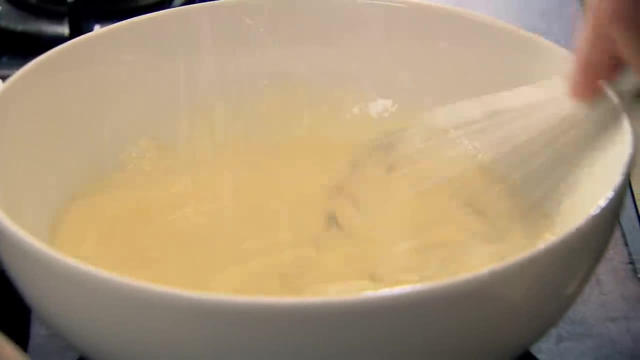 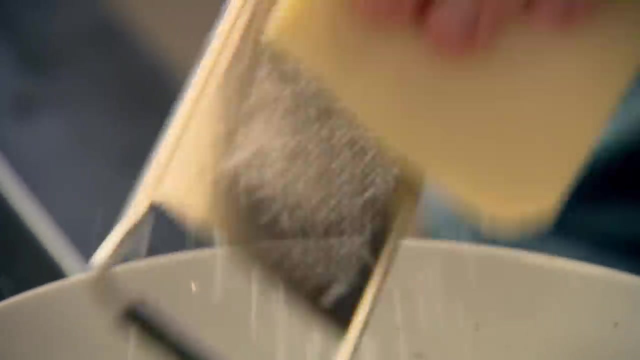 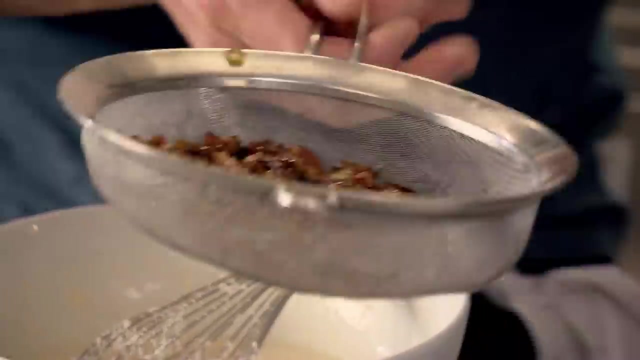 and one-third of the savoury custard, A touch of salt, A touch of pepper. I'm going to grate some gruyere cheese That makes a really nice sort of creamy, less of an eggy quiche. Take my amazing crispy pancetta and leeks in. 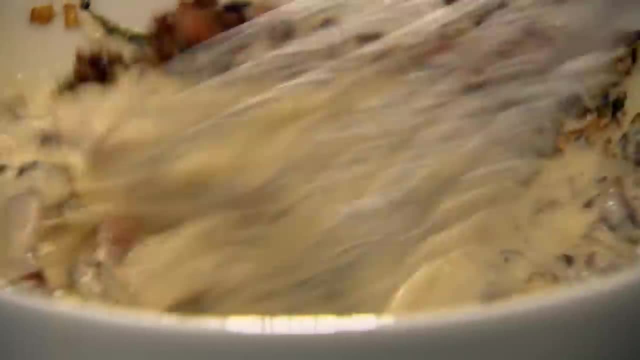 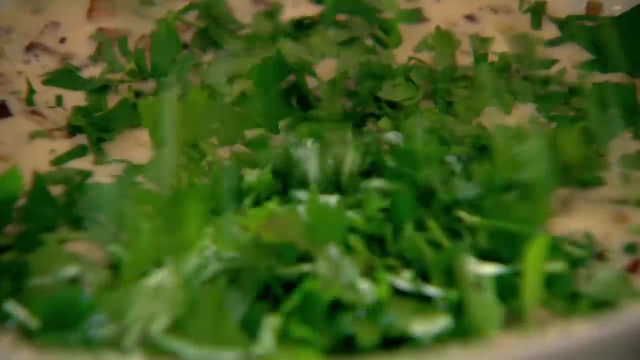 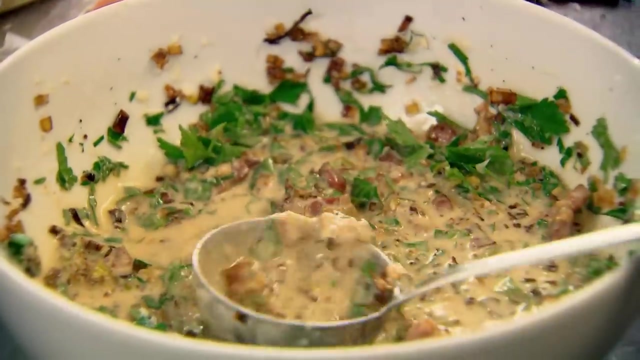 Mmm, Give that a good mix. Needs one more little thing: Some freshness. Flat leaf parsley- Incredible, Really important. Just a taste, Mmm. The mixture With the quiche filling ready. next finish off the pastry. 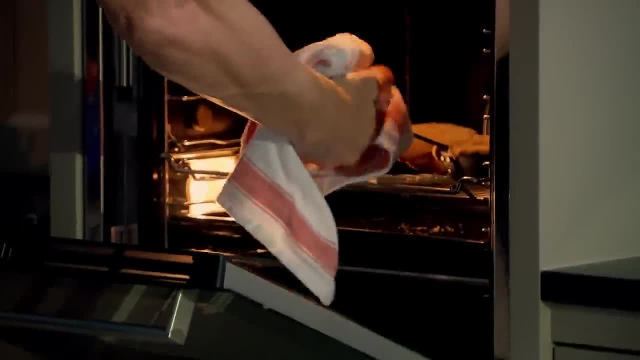 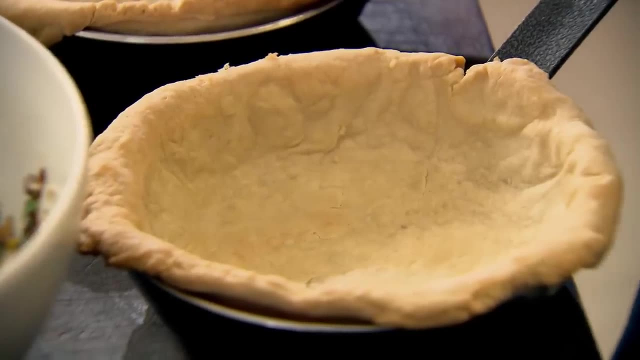 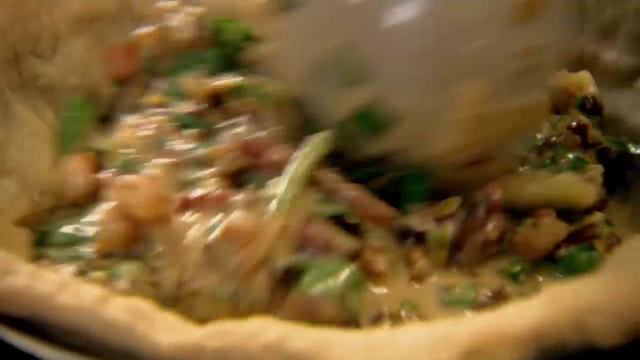 Remove the fallen weight and return to the oven to get it lovely and golden all over. Now, when we fill them, give that a really good mix-up: Beautiful Grate over some more cheese, which will bubble up and melt beautifully And then into the oven. 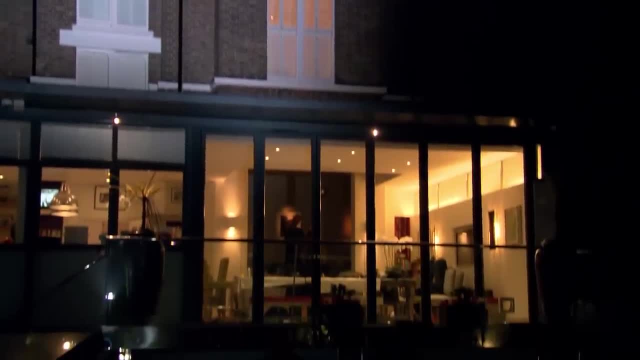 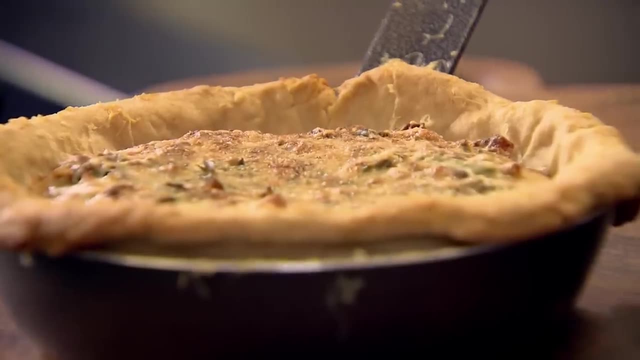 Bake your quiche for 15 to 20 minutes- Incredible. It's got that nice sort of cheese-on-toast smell from the top. It's sort of baked. But the secret of any good quiche is in the short crust, because that's the hero. 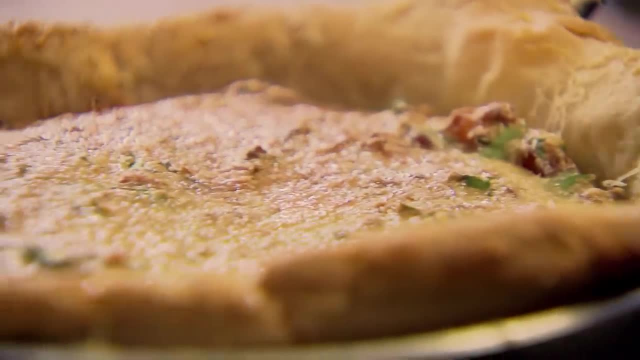 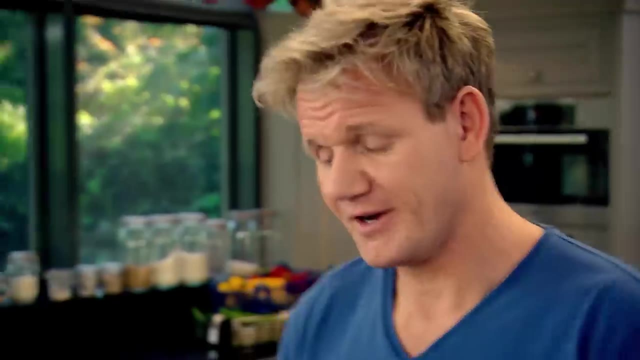 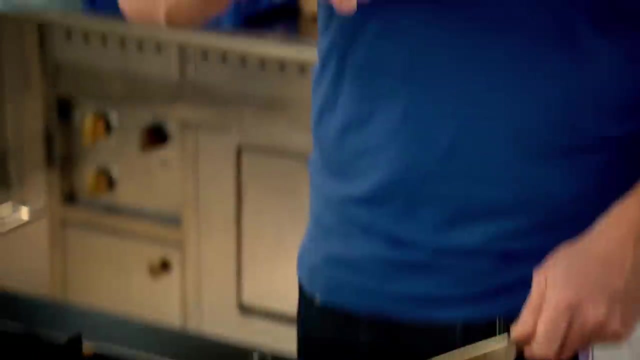 Really important to put the water on first, so you can just have it gently simmering away ready for the pasta While the water comes to the boil. start the sauce by slicing mushrooms. First off fingers, One in front, two behind. 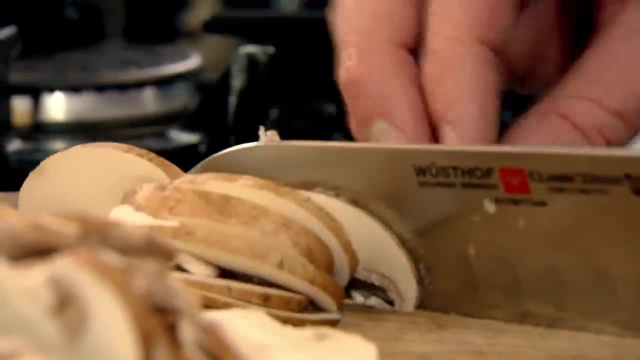 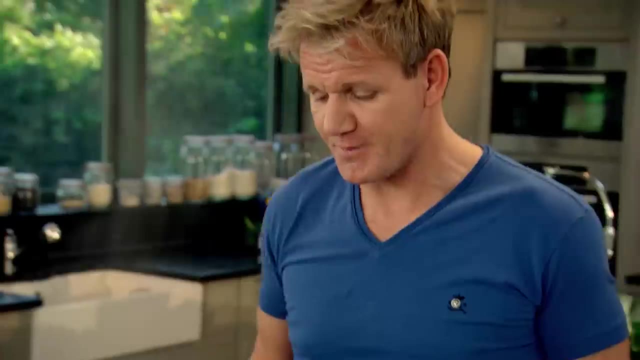 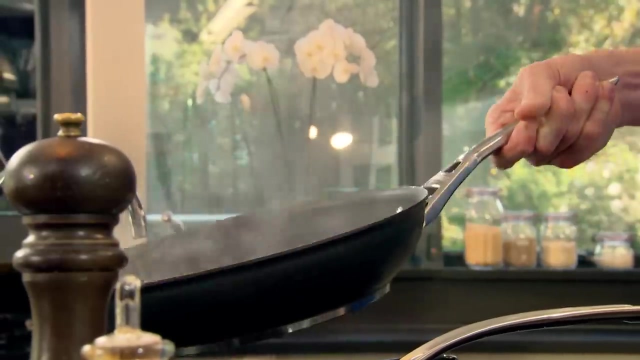 Up and down. Then add olive oil to a hot frying pan. I want that nice colour on the mushrooms. Off the heat Literally ten seconds, And when you toss something really important, to get all the ingredients at the end of the pan. 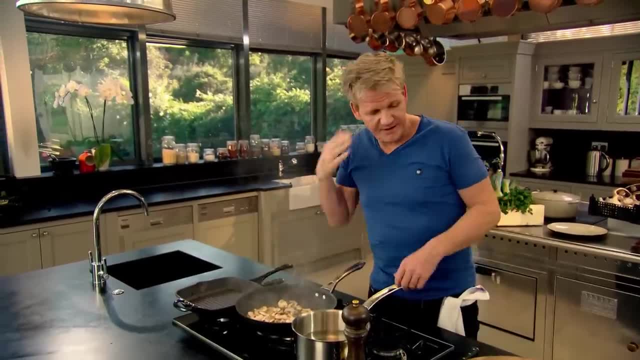 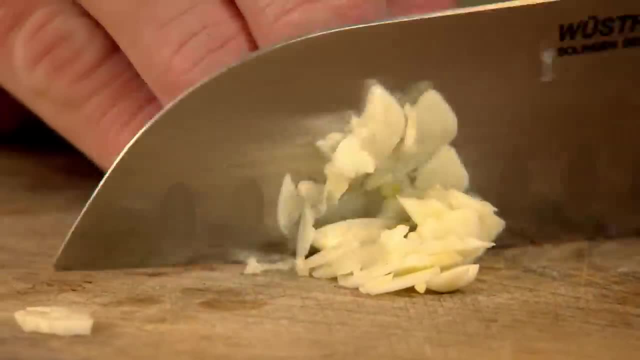 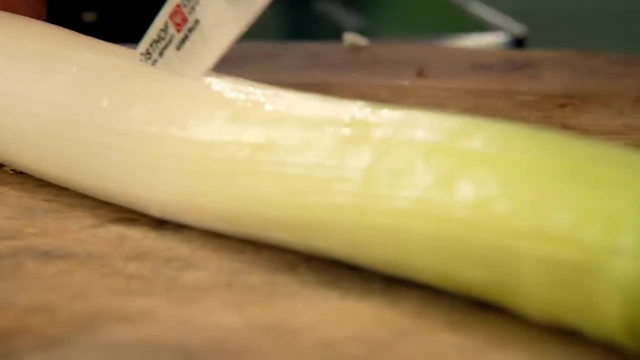 Push down and pull back. That noise that That's all the water coming out of the mushrooms. Next, finely chop a fat clove of garlic. Then prepare your leeks. Just take your knife and go down through the centre, Turn it over. 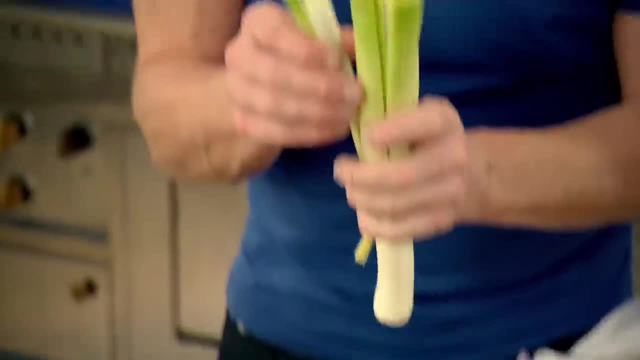 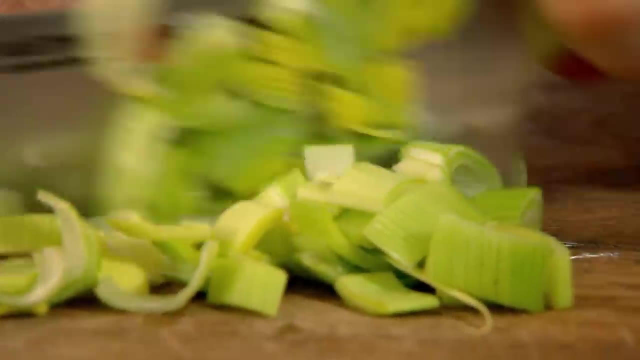 And again into quarters. So you've got all that opening up And then just rinse the top of that to get rid of any potential dirt or sand. It just breaks up into nice little quarters. Add all that leek into those mushrooms. 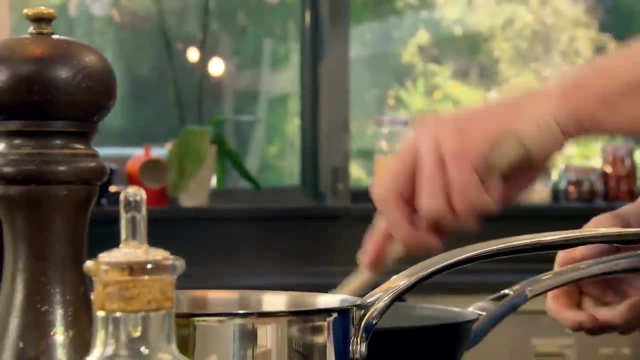 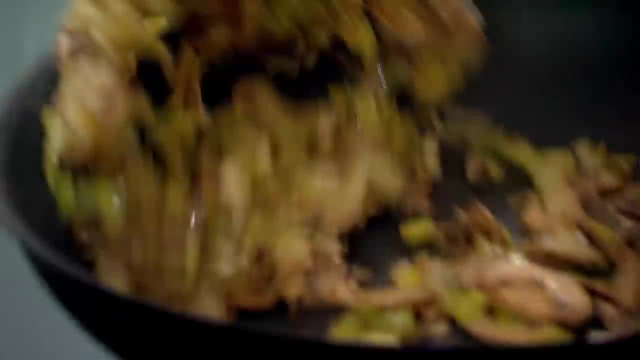 Beautiful. And now the secret is to get rid of that water inside the leek As it cooks down. all the water's gone. You've just left that really nice, intense flavour. Garlic's gone, nice and crispy. Now we're going to add a touch of chicken stock in there. 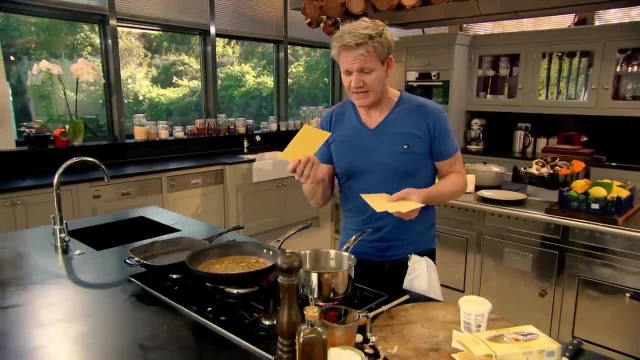 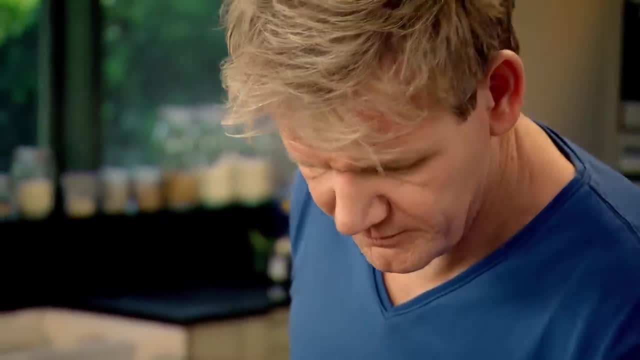 Mmm, Beautiful Lasagne sheets. Just going to drop the sheets into the water. Lasagne sheets are an unusual choice for a dish like this, But they work brilliantly, Although any type of pasta you've got in the cupboard will do. 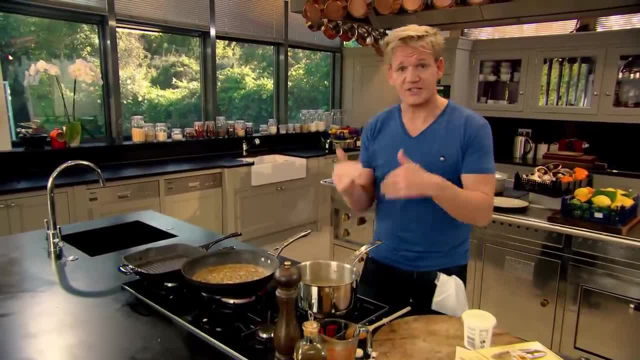 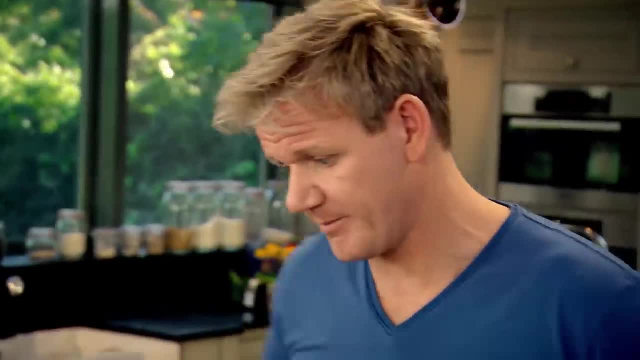 And just twist that pan. That stops any pasta actually sticking to the bottom of the pan. Chicken stock will reduce down by half And it almost delays the bottom of the pan Basically washed all that wonderful flavour. Turn the gas down And add a couple of tablespoons of cream. 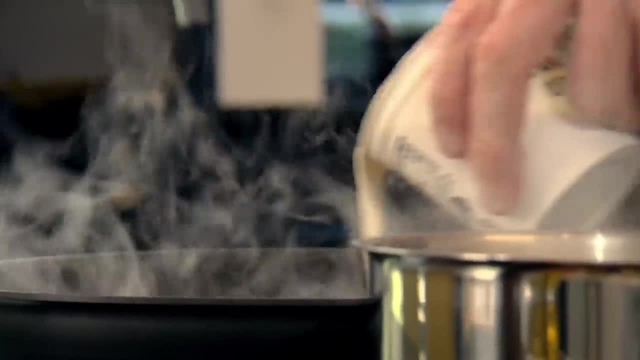 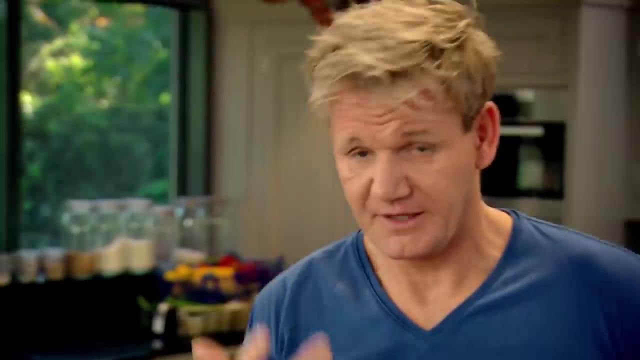 This just enriches the dish. Bring it back up to the boil And let it simmer for three to four minutes. Now the secret of the pasta is just taking it out a little early. So you've got that nice texture. Hold up the sheet and just nip it.